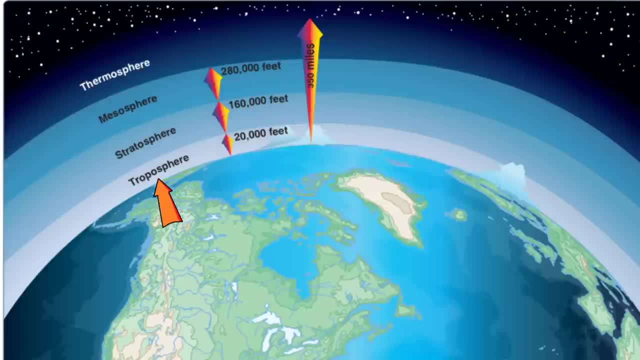 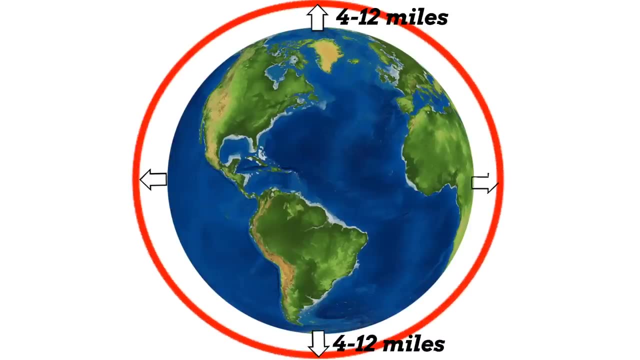 that we're talking about, Because that's where the majority of weather takes place. Now, at the poles, the troposphere starts at the surface and goes up somewhere between 4 and 12 miles Over the equator. it only goes up to about 48,000 feet, And above that there's a thin 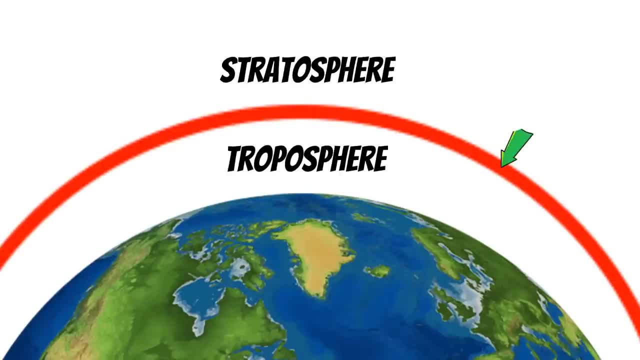 boundary layer between the troposphere and the stratosphere, called the tropopause, And this boundary layer traps most moisture and weather inside of the troposphere, and that's why there's really not a need to study the other layers Inside the troposphere for every. 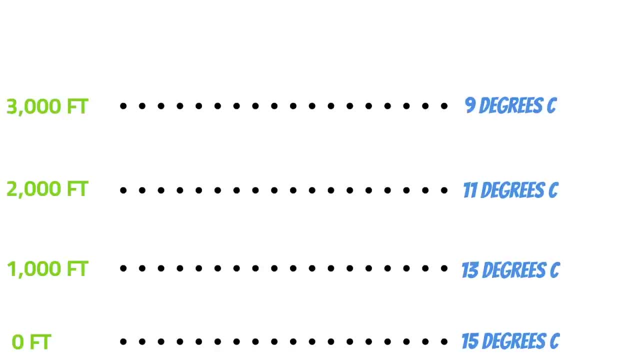 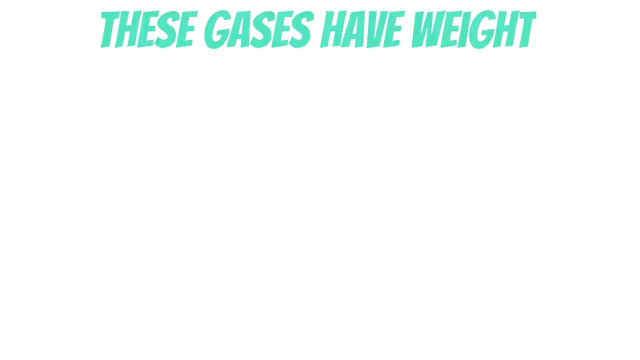 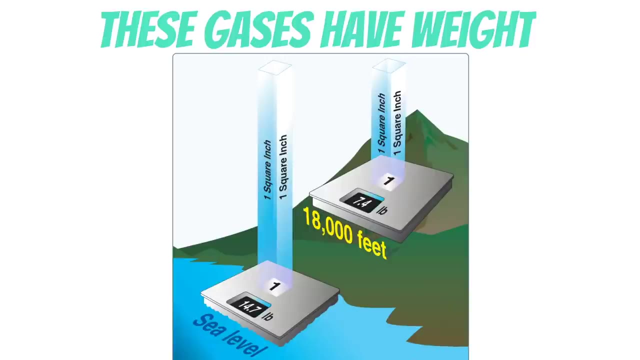 thousand feet of altitude that you gain, the temperature decreases about two degrees Celsius. Now, oddly enough, even though they're invisible, all these gases in our atmosphere have weight. In fact, our atmosphere is 350 miles high, and if you were to weigh a one square inch column of air, 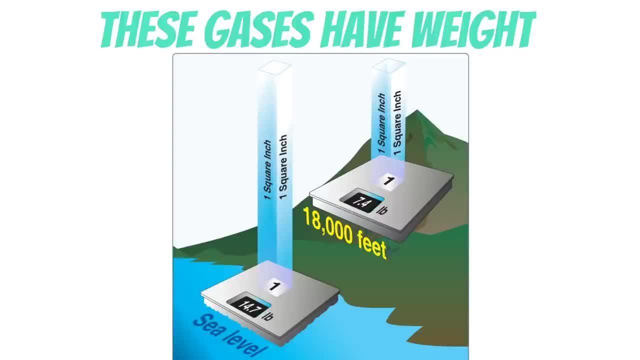 the whole height of our atmosphere. it would weigh 14.7 pounds, And as you increase your altitude, there's less air on top of that other air, so it would actually weigh less, And this is why air pressure decreases as altitude increases. 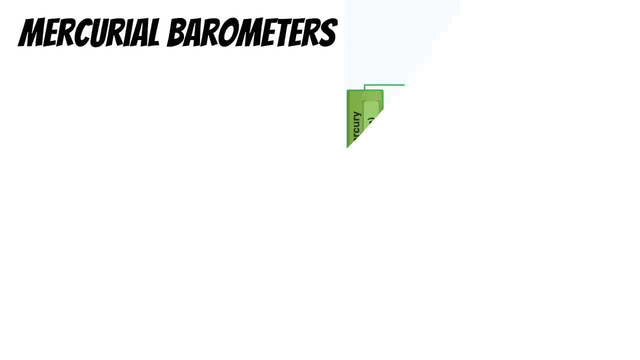 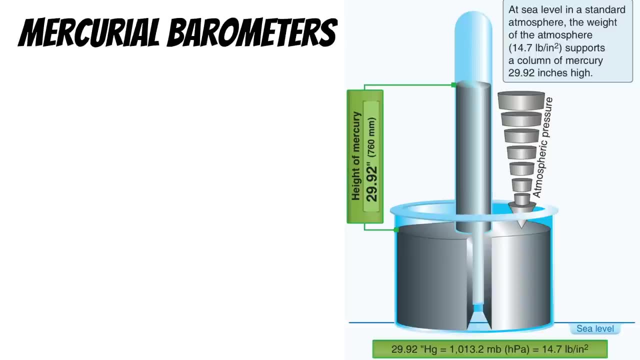 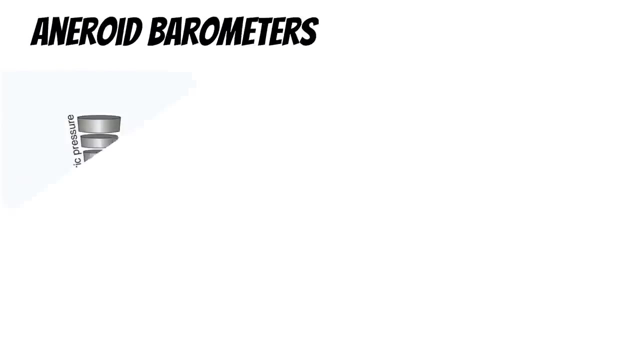 To measure air pressure we used to use mercurial barometers And at sea level, on the average day, the air pressure would push the mercury up to 29.92 inches, And this is where we get that standard pressure setting. Today we use aneroid barometers to do that instead. They're not quite as accurate. 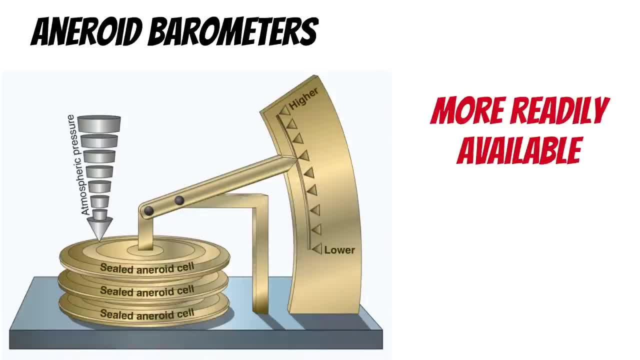 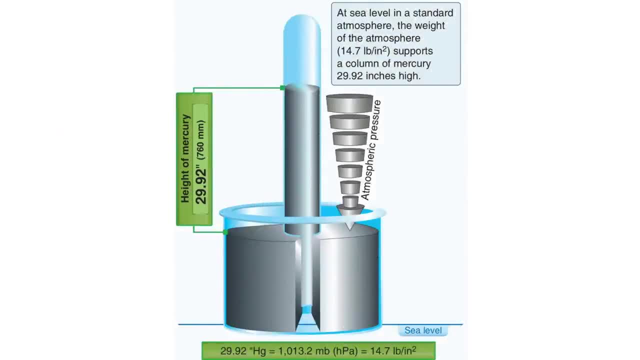 but they're a lot more readily available and they're probably a little bit safer. Now, as I mentioned a second ago, our standard air pressure at sea level is 29.92 inches of mercury, but in some countries they measure pressure in millibars instead. If you're lucky enough to be on the metric system. the standard pressure in that case is 1013.2 millibars. Anyways, for every thousand feet of altitude that you gain, the air pressure decreases about one inch of mercury, or roughly 34 millibars. Now let's go back and talk about the atmosphere for just a little bit. 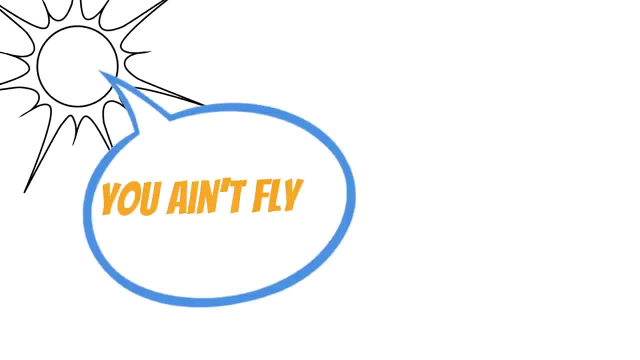 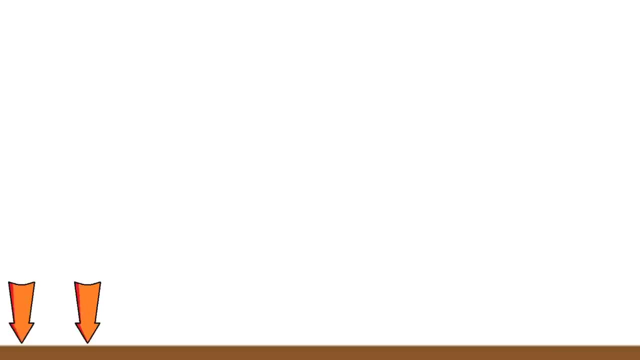 As you probably already know, the sun is responsible for the majority of our weather, and it's mainly because the Earth's surface is heated by the sun unevenly. When the Earth's surface is heated, this causes the air near the surface to also be heated, And when this happens, the air 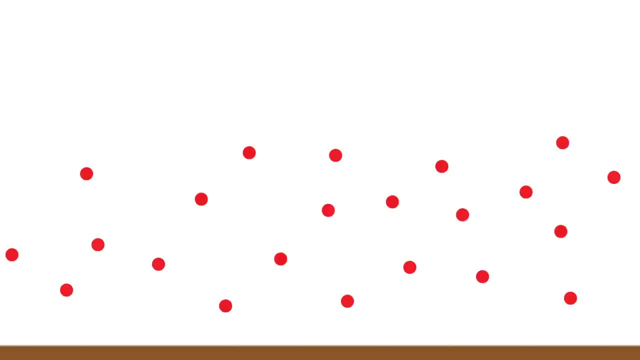 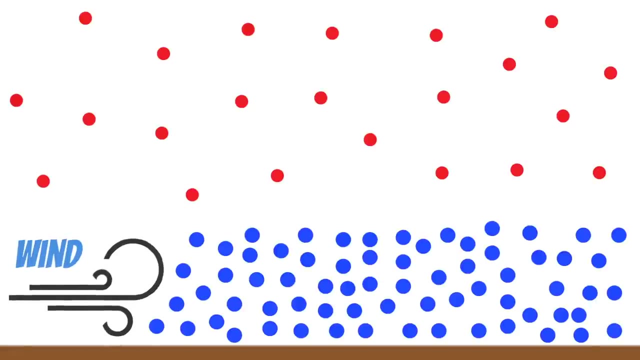 molecules in this air spread apart and the warm air gets less dense. That causes the warm air to rise and it gets replaced by cooler air, as it does. If you haven't already started flying, this is one of the first things you're going to notice. if you fly on a 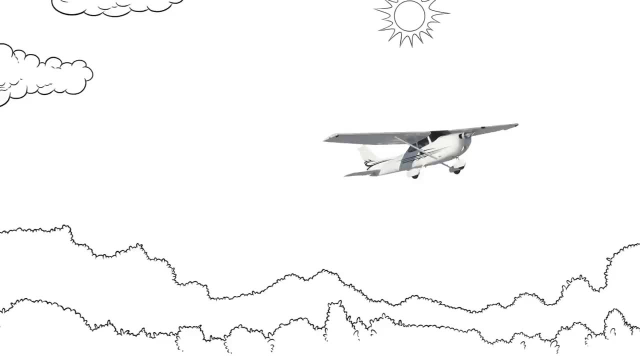 sunny afternoon You're going to feel those updrafts, push your plane around quite a bit, especially if you're somewhat close to the ground, And some types of ground heat up more quickly than others and water heats up a lot less quickly than the ground And because of that those updrafts. 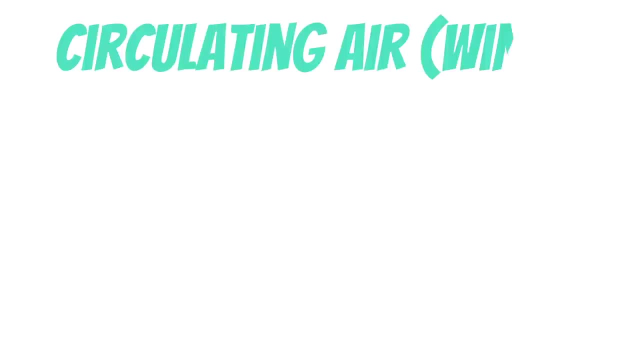 won't be nearly as bad over water. So now what we get is a bunch of air circulating in our atmosphere. That warm air rises and the cooler air rushes in to replace it, And that's what causes our atmosphere to be in constant motion. Now, as I just kind of touched on, 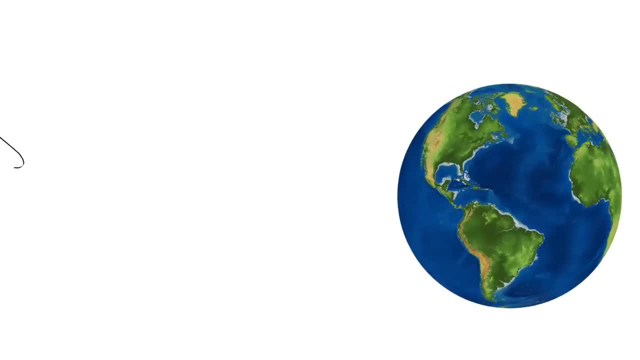 the sun heats the ground unevenly, but it also heats the entire earth unevenly. In fact, the equator takes most of the direct sunlight and the poles receive very little Because of that. if the earth didn't rotate, this is what the majority of that airflow might look like. 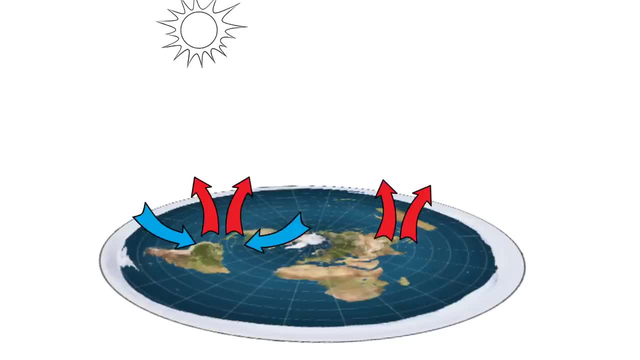 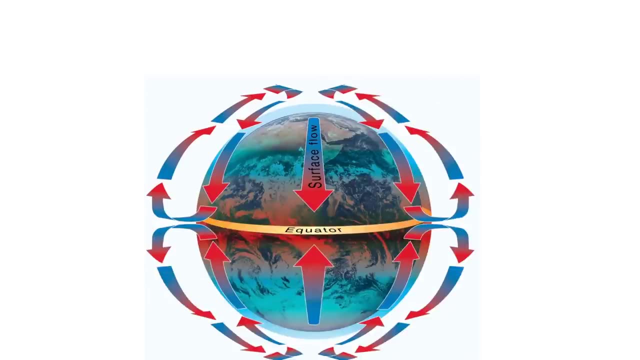 For my friends who believe in a globe of this shape, this is probably what that circulation looks like for them. Sorry, I can't help myself. I just find flat earth stuff funny. Anyways, we're going to focus on the ball earth theory, because that's the way the FAA explains it. 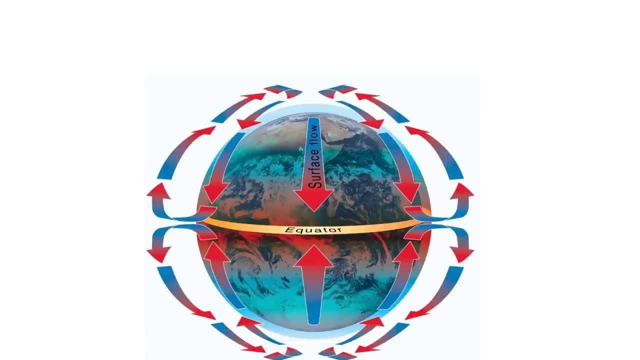 in the pilot's handbook of aeronautical knowledge, At least for now anyways. So, as we mentioned, if the earth didn't rotate, the flow of the warm and cool air would look something like this: But because the earth rotates, the Coriolis force forces these airflow. 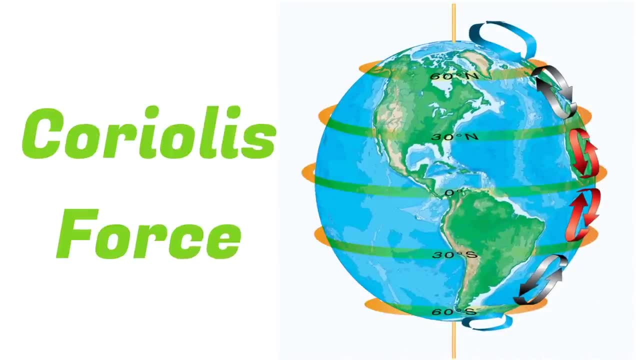 patterns to look more like this: Let's spend just a minute talking about the Coriolis force, And I want to do that because to me it seems like the Coriolis force works backwards And I feel like if I don't explain this very well, this next part's not going to make very much sense To do that. 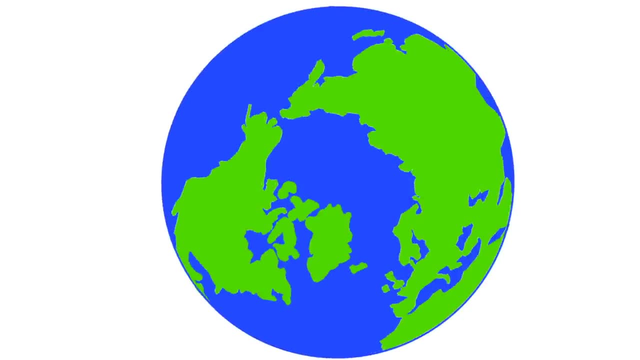 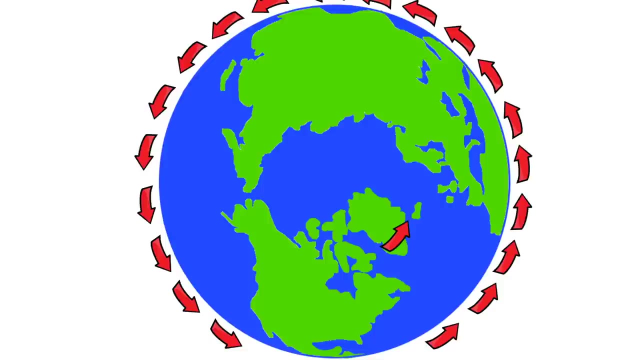 I'm going to take a look at the earth from the top of the globe From up here. the earth rotates counterclockwise on its axis. As you can see from up here, everything out here by the equator has to travel a longer distance than anything closer to the poles. Because of that, everything out here, 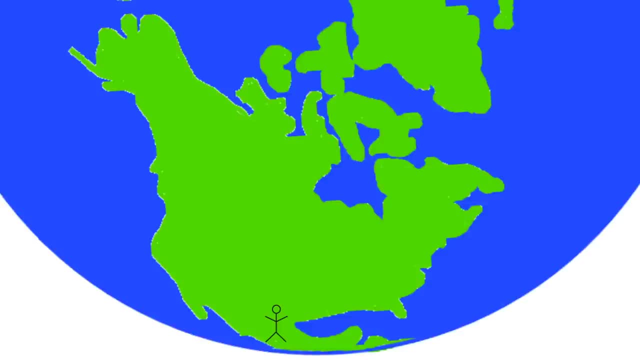 closer to the equator travels just a little bit faster. Now, let's say I'm standing here in Mexico and I could throw a baseball all the way to the North Pole. Not only would the ball be traveling north, but it would also be traveling in the same direction as the rotation of the earth. 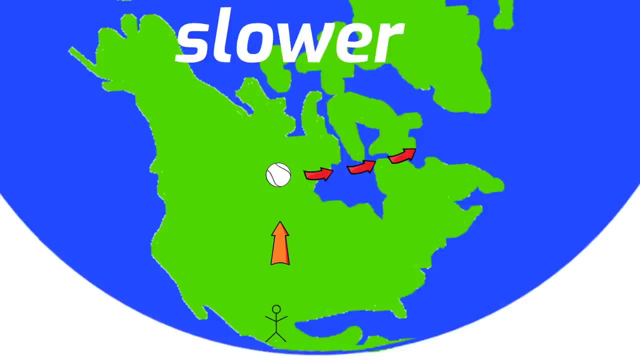 But as the ball moves north, the earth will rotate in the same direction. As the ball moves north, the earth beneath it actually moves slower And because of that, as it travels north, it also moves to the east, And that's because it was already moving east, but now it's moving east. 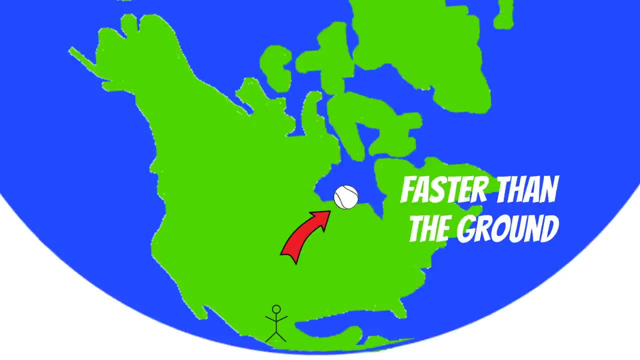 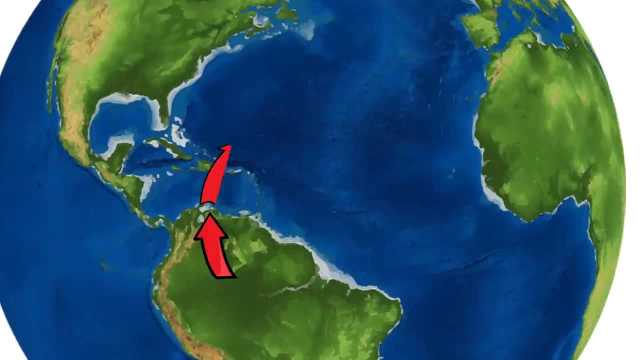 faster than the ground beneath it. And that's the Coriolis force in a nutshell. And just like my baseball, when that warm air at the equator rises, it travels north, And when it does, it's slowly deflected to the east And it only makes it up about a third of the way. 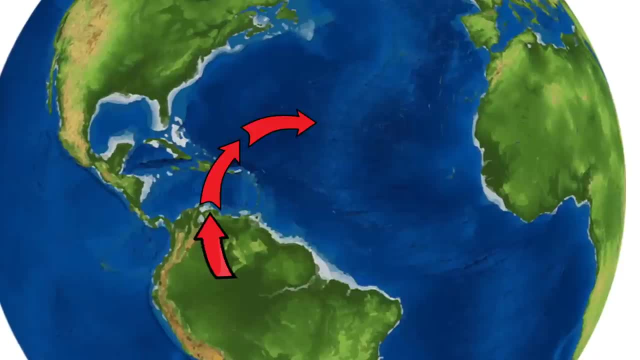 before, the air is completely moving east, And this is actually why the upper level winds in the continental US are usually out of the west. While all this is happening, this air begins to cool down. This causes the air to become more dense, And when it does, it sinks back down to 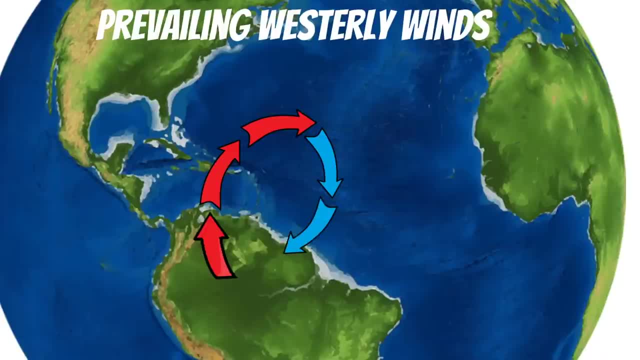 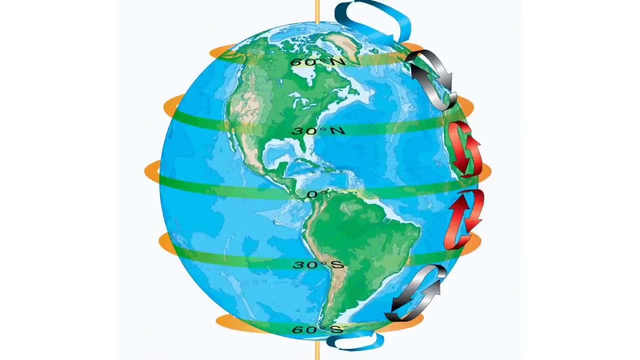 the surface. Once it does, it moves back to the south to take the place of the warm air In the southern hemisphere. the air moves in the opposite direction And really similar cycles occur between the 30th and the 60th parallel and up at the poles. Now, 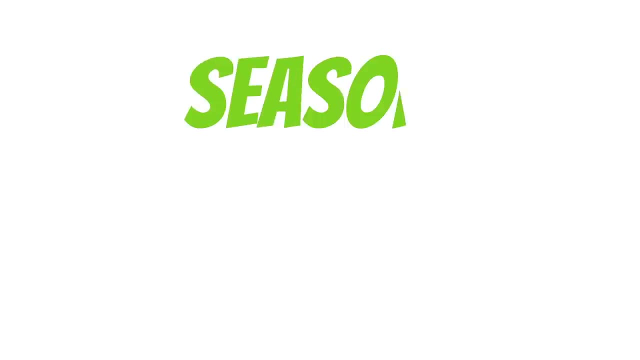 things do get a little bit more complicated when we start talking about the seasons and the fact that the continents heat up more quickly than the oceans do. We'll talk a little bit more about those here in just a minute. But you should be aware that friction caused 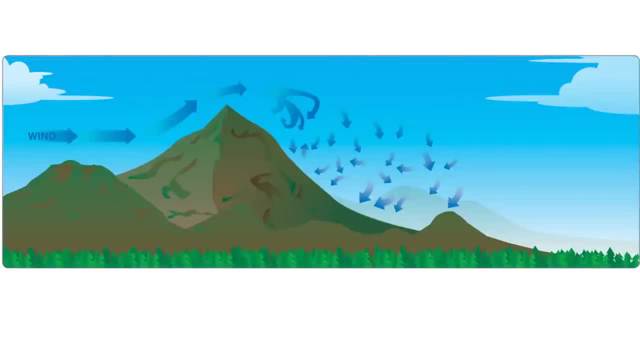 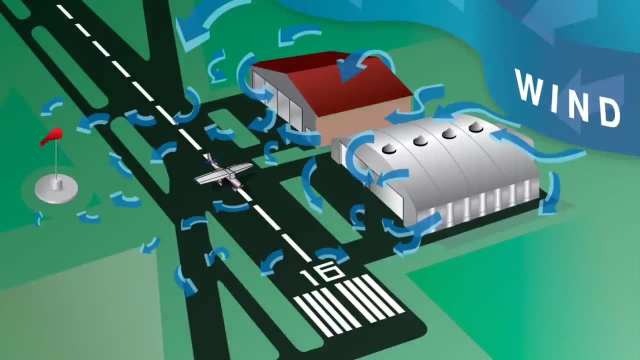 by the topography of the earth also comes into play And, as you can see from this picture, this can be anything from mountains, hills, rocks and trees to man-made features like buildings or even hangars, And all this stuff can cause changes in the wind direction. wind speed. 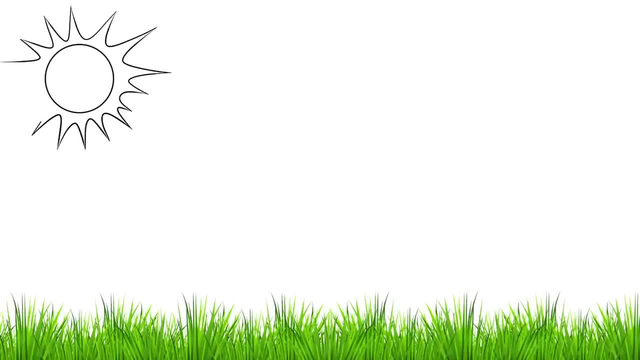 and also cause gusty winds. Okay, so now we know that when the sun heats the ground, the air above the earth is heated, And when the temperature changes, so does the air pressure, because those air molecules spread apart. Not only is the air pressure lower now, but there's also more room. 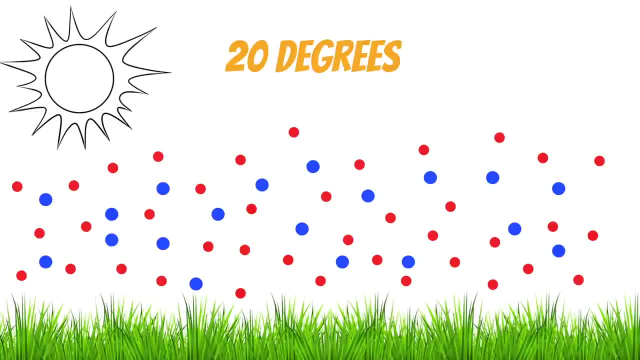 for water vapor. In fact, for every 20 degrees increase in temperature, the amount of water vapor that the air can hold actually doubles, And water vapor is lighter than air, so this can make the warm air rise even more quickly. We'll talk about this more in just a minute, But for now just. 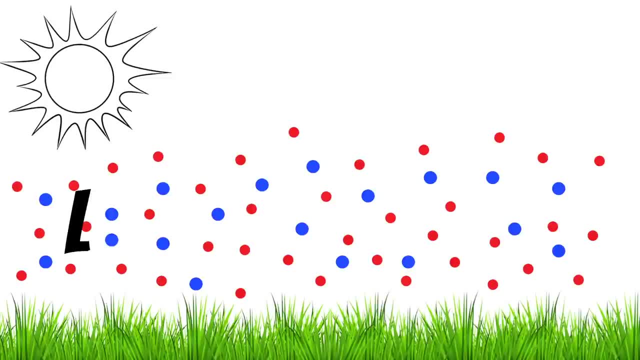 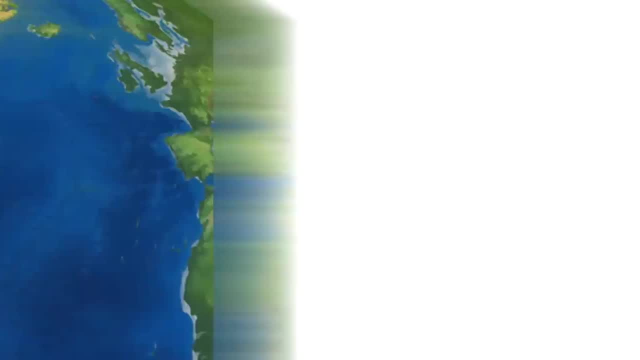 realize that with all these areas of different temperature, we also get areas of different air pressure, And because of that now we have areas of high pressure and areas of low pressure. With that in mind, air always moves from areas of high pressure to areas of low pressure. 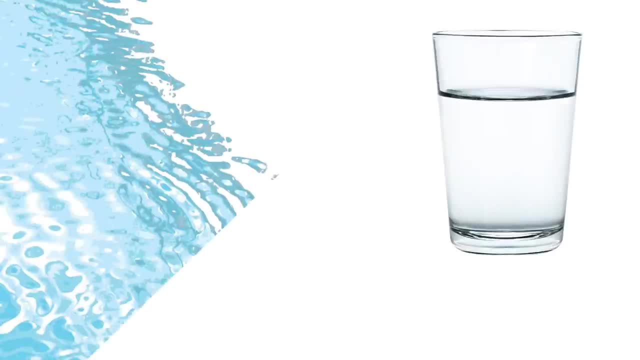 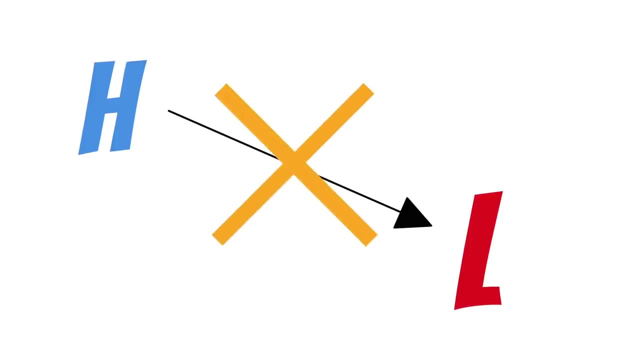 Think of a glass of water. If I pour it out on the ground, it's going to move to the lowest spots in that area. But oddly enough, the air doesn't move in a straight line to these low pressure areas because of the Coriolis force. Remember, high pressure air is cooler air. that. 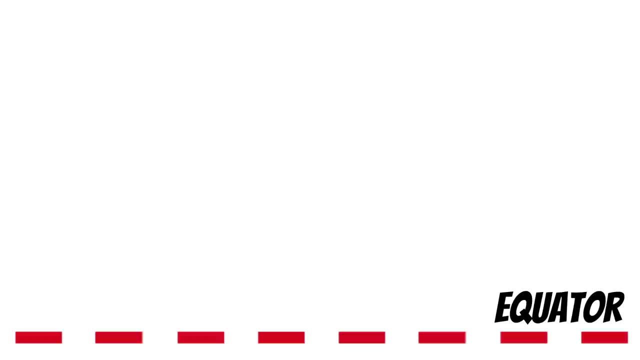 is sinking back to the surface. So in the northern hemisphere the air doesn't move to the south. The northern parts of the sinking air are deflected to the east And any air that moves to the south is deflected to the west. So because of that, air actually moves around the high 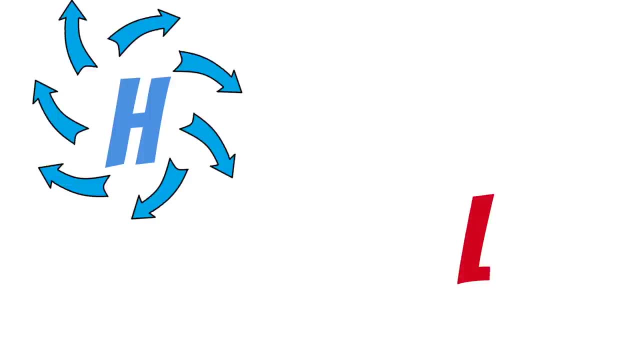 pressure system in a clockwise motion. Areas of low pressure are those areas where the warm air is rising. So as that air rises, it also deflects to the east And this causes a counterclockwise movement of that air. But the closer the air is to the surface, the straighter the air travels to. 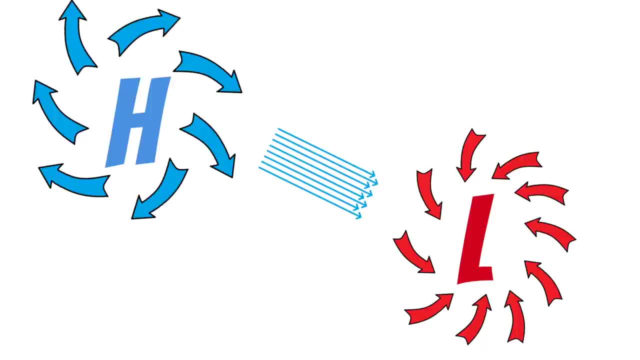 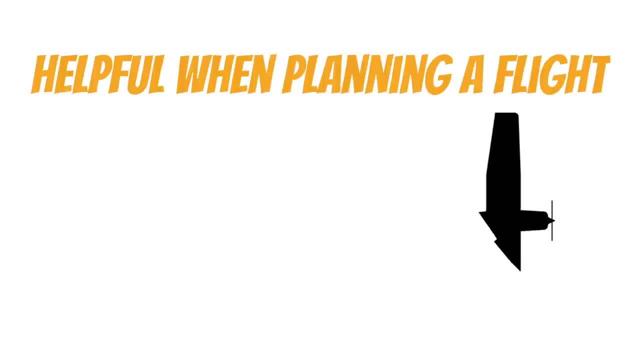 that low pressure area because of the friction on the ground. So now you're probably wondering why you need to know this as a pilot, And the first reason is that this can be really helpful when you're planning a flight, because it can help you pick a flight path where the winds are more. 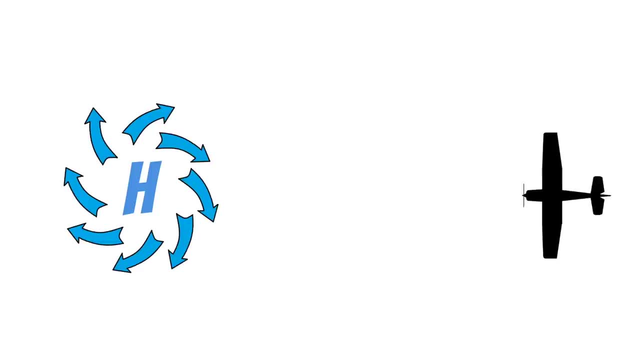 favorable. For example, if I know that I'm flying near a high pressure system, would I want to fly north or south of it? Well, in this example, we want to fly south of it because we're flying westbound. This will give us a tailwind, which will actually increase our ground speed, And 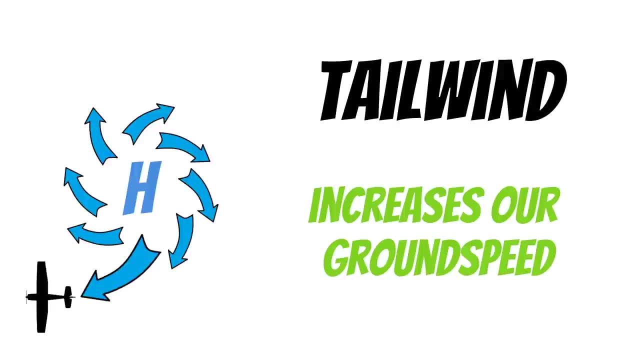 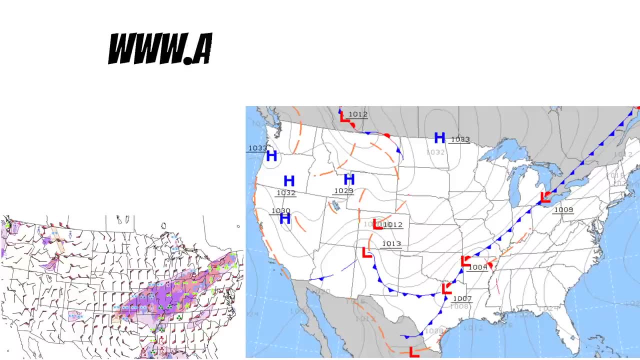 that's going to help us get to our destination even faster. Now we can get an idea of how strong these winds are. one of two ways. Let's pull out a couple weather charts from aviationweathergov. Now, if you have ForeFlight, you can actually look at these charts in there as well. ForeFlight. 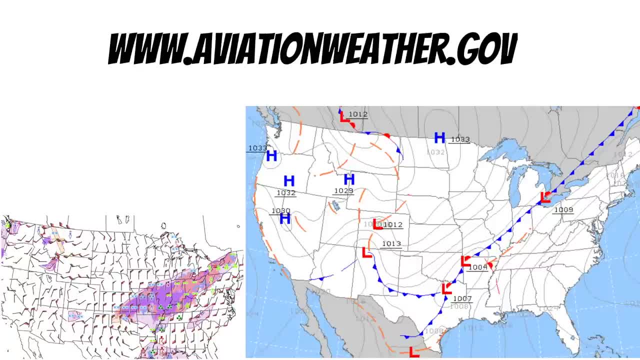 makes everything so easy these days, because almost everything you need for flight is in one spot. But if you don't have ForeFlight, this is where you should be checking the weather, because this is probably the best weather source available for pilots. First things first, let's take a 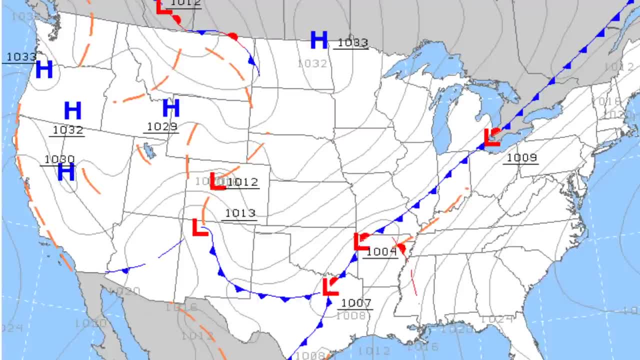 look at this prog chart. This one is an analysis of the surface conditions. As you can see, we've got some high pressure areas here and some low pressure areas, So we know roughly which direction the wind will be moving at altitude. But notice these lines surrounding. 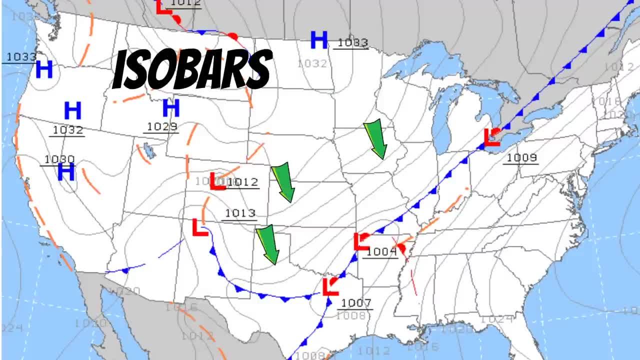 the pressure systems. These lines are called isobars and these represent how much the pressure is changing in these areas. This is important to you because the closer these isobars are together, the windier it is in these areas. Because of that. 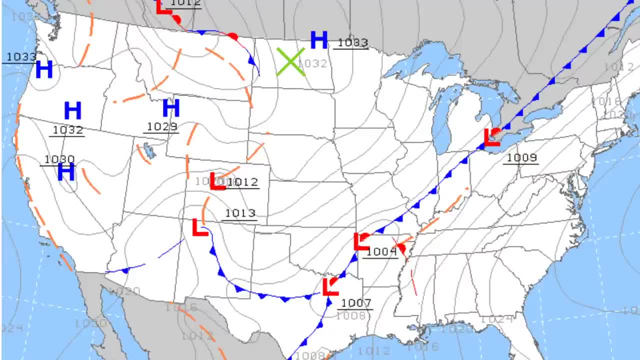 I know that if I'm flying here in North Dakota I should have less wind than normal and it should be from the south. Down here in Northeast Oklahoma it's going to be super windy and the wind should be coming from the northeast The other way we can see. the wind conditions are on these weather. 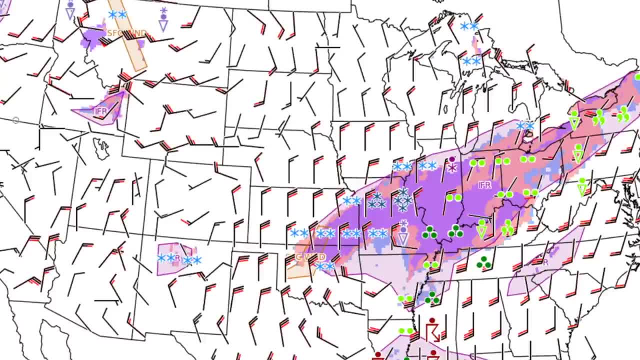 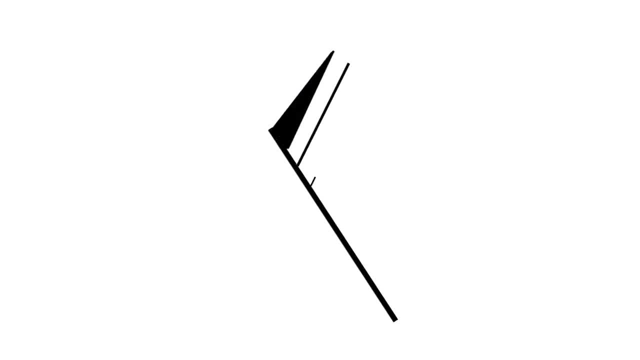 charts that depict wind flags. This particular chart is a surface weather chart. Now, to me, these little wind flags work backwards. The side with the flag is the side where the wind is coming from. Short bars represent the direction the wind is coming from. So if I'm flying here in North, 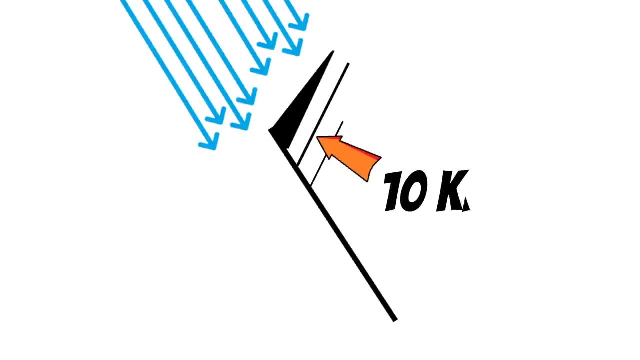 Dakota, I should have less wind than normal. So if I'm flying here in North Dakota, I should have less wind than normal. Long bars represent 5 knots of wind, Long bars represent 10 and the triangle represents 50. And you have to add all these up to get your total wind speed in this area. 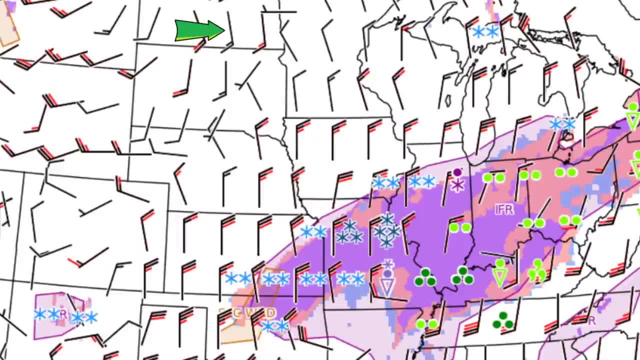 So, as you can see here, we have south winds at 15 knots in North Dakota. as I mentioned before, It looks like winds are almost straight out of the north at 20 knots in Oklahoma, And that's probably because there's a cold front that just passed to the southeast. 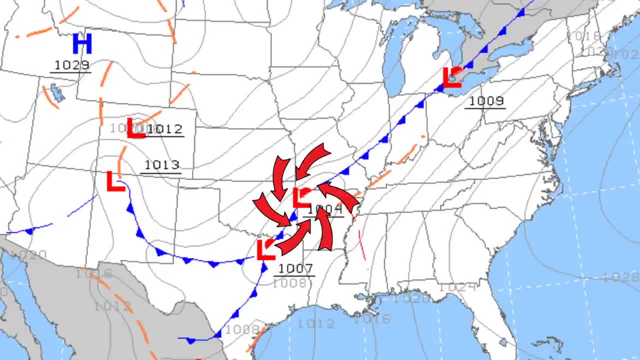 Otherwise, that wind should have been more out of the northeast. We'll talk more about that in a minute, But before we do I just want to mention something else about these pressure systems that I think is important When you think of high pressure areas. 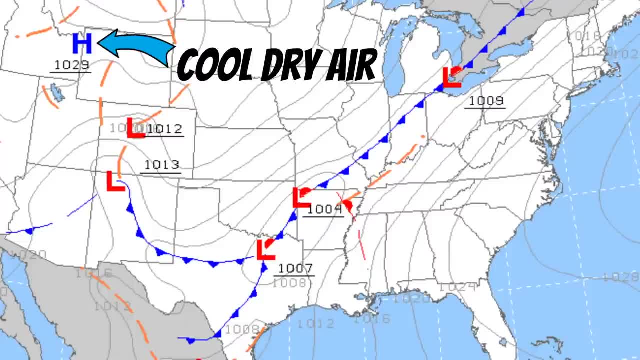 remember these as areas of cooler, drier air that drop back down to the surface. This drier, heavier air is much more stable, so you're typically going to see good weather in these areas. Now think of those low pressure areas as that warm air that rises. 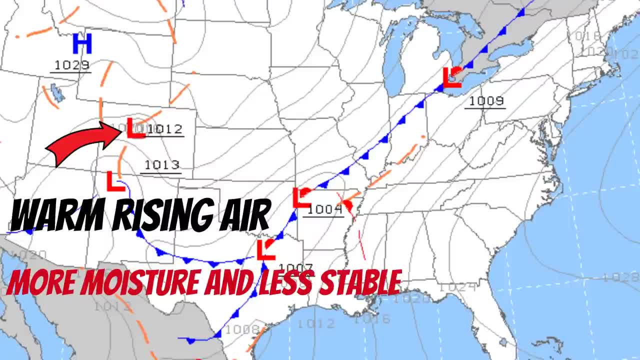 It can hold more moisture, so it brings the water vapor up with it, which causes clouds, rains and all kinds of other bad weather, And this is going to come back into play in just a minute, But for now let's talk about fronts. Okay, so we've already discussed how the sun 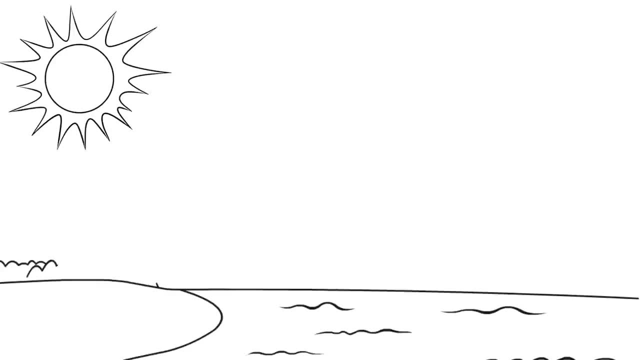 heats the different types of ground unevenly, and how water and land heat differently as well, And this causes air circulation in a lot of areas across the globe. But there are also a lot of areas on our planet where the surrounding ground and water is very 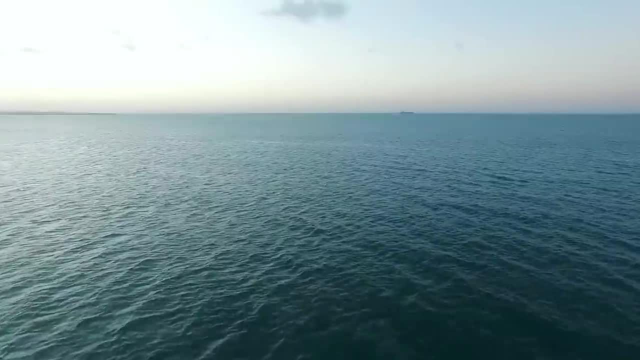 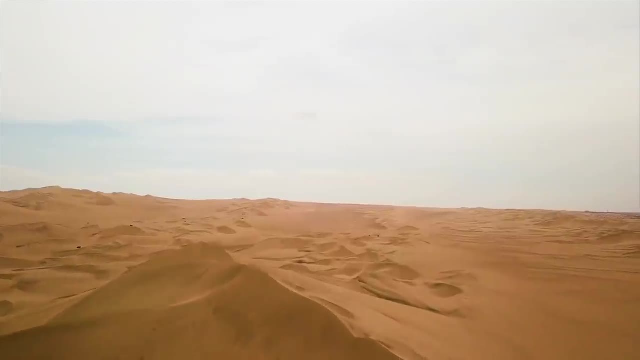 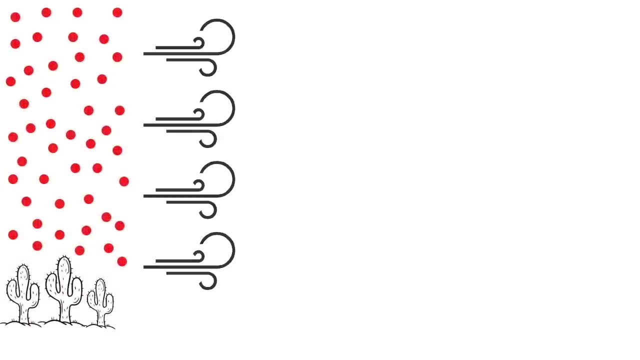 similar, And these stagnant areas occur in polar regions, tropical oceans and dry deserts. These areas don't circulate that much. These become stagnant areas of either cool air or warm air. The air in these areas build over time and they eventually push their way into other regions. 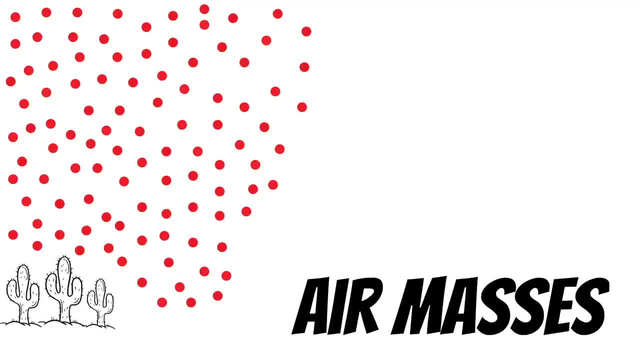 These are what we call air masses. As these air masses move forward, there's a boundary layer that forms between the air mass and the air in front of them, And this boundary of changing air is called a front. The front at the beginning of a warm air mass is called a warm front. 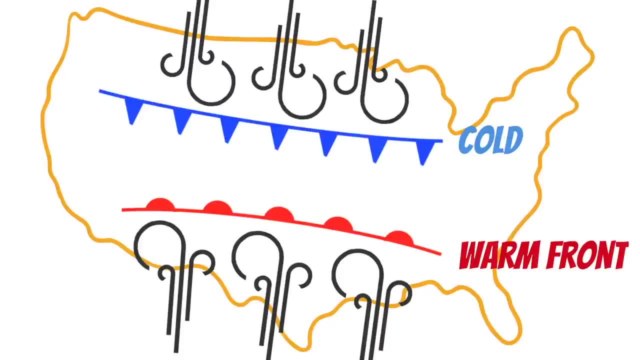 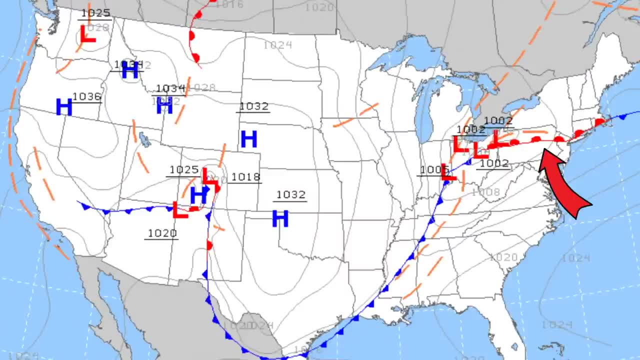 and the boundary at the beginning of a cold air is called a cold front. If we take a look at our weather charts, we can see the different types of fronts moving into our area. Warm fronts are depicted as these red-hot blisters, while cold fronts are depicted as these cold blue icicles. Now, on occasion, you will see two other. 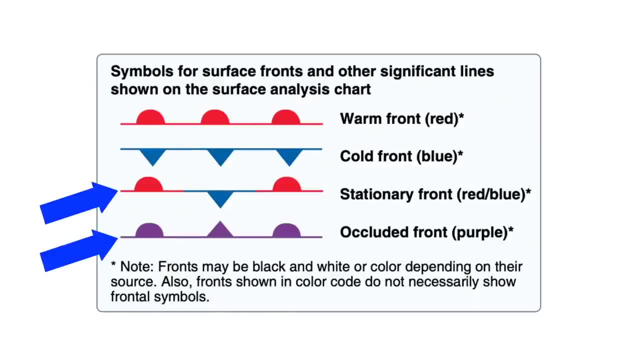 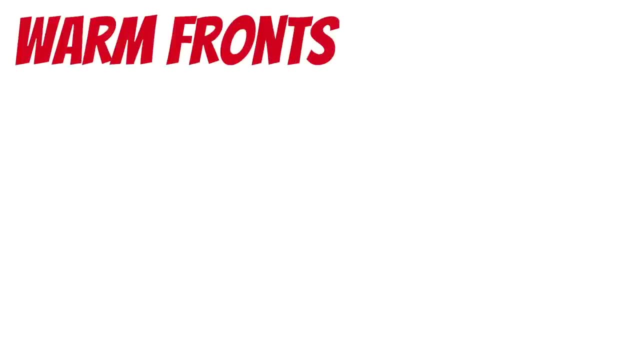 types of fronts. These are occluded fronts and stationary fronts, and we'll talk more about those here in just a minute. Let's start by talking about warm fronts first. Warm fronts are very slow and only move about 10 to 25 miles an hour. The warm air tries to push into the cooler air. 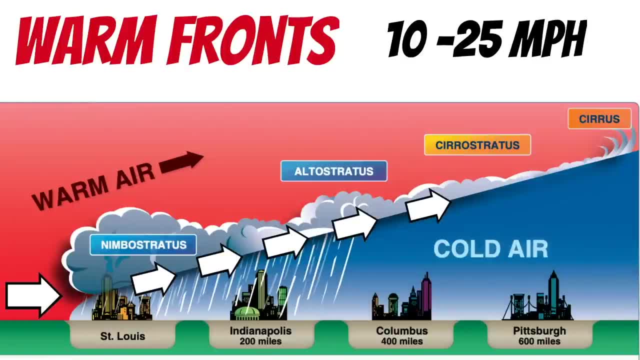 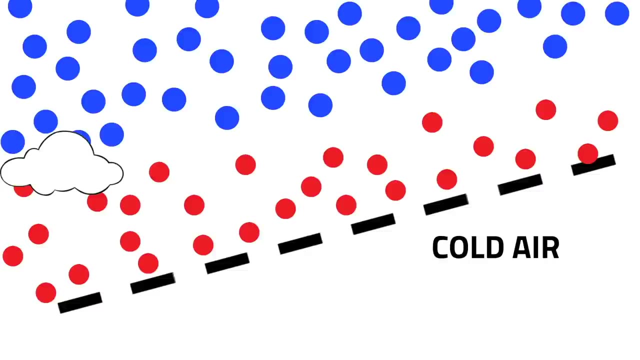 but because it's lighter, the warm air is also pushed up above the cooler air in the process. Now, as I mentioned earlier, warm air can hold more water vapor, so warm fronts will typically bring a lot of humidity into the area. As this warm air rises, the temperature drops, and when 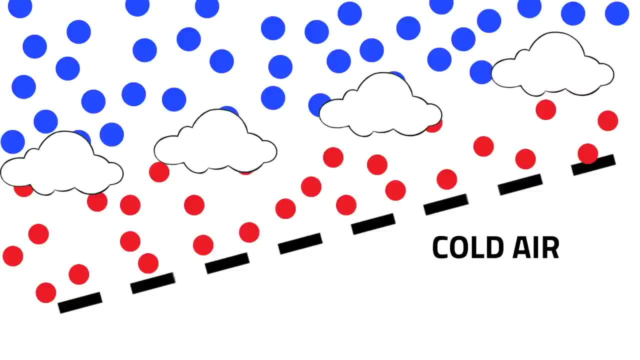 that happens, you get condensation. Let's stop right here for a second and go into a little bit more detail about this, because warm fronts are typically more humid than cold fronts. Once you understand a few basic things, you'll understand what kind of weather you can expect. 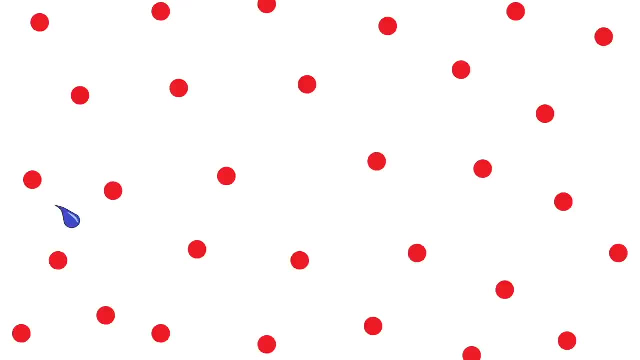 when a front passes. Now, if you remember from earlier, the air in our atmosphere actually has water vapor in it, and the warmer it is, the more water vapor the air can hold. This ratio of water vapor in the air to how much it can hold is called relative humidity, and dew point is a specific. 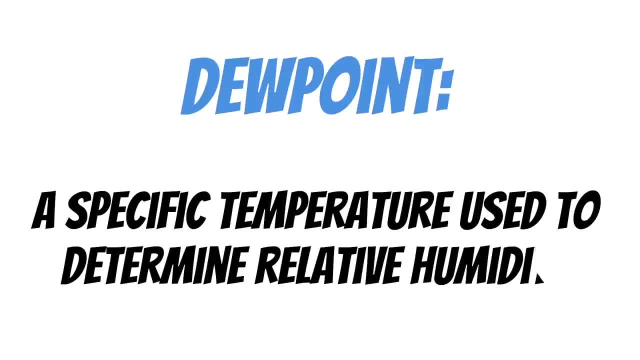 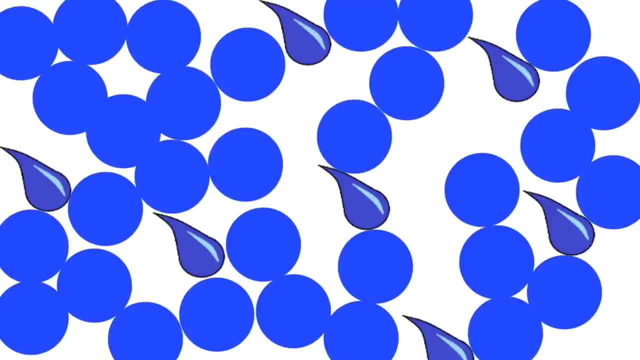 temperature that we can use to determine our relative humidity. Let's say the dew point is 14 degrees Celsius. When that air is cooled to a temperature of about 15 degrees Celsius- the temperature of 14 degrees- the air becomes completely saturated and it can't hold any more. 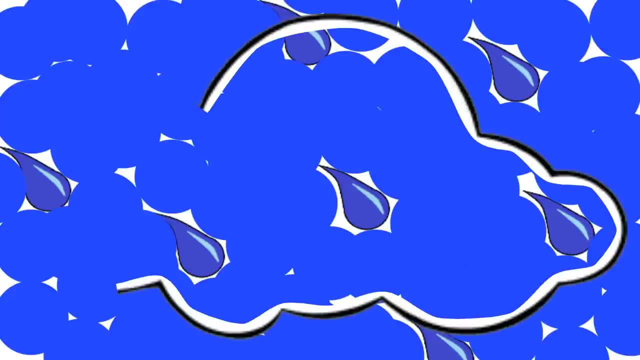 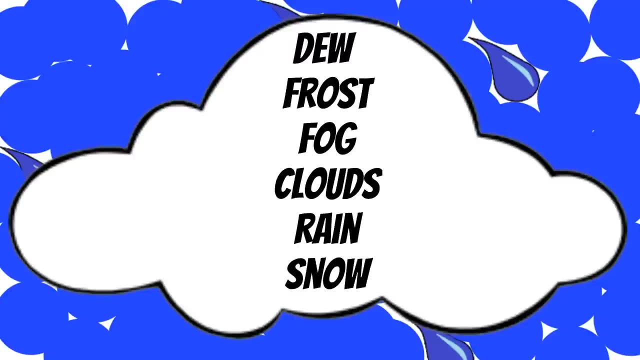 moisture, And because of that, moisture begins to form in the air, and this can take the form of dew, frost, fog, clouds, rain or snow. Now, as we already mentioned several times, when air is heated, it rises, And in the beginning of the video we also mentioned that the temperature drops. 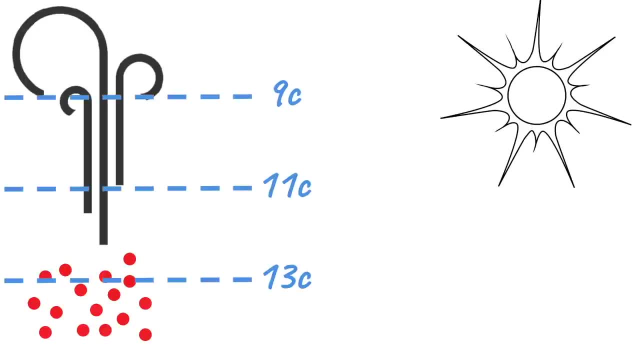 2 degrees Celsius for every 1,000 feet of altitude that you gain. And as that warm air rises, it also expands, because that air at higher altitude is less dense. And as that warm air expands, this also causes the temperature to drop. And how? 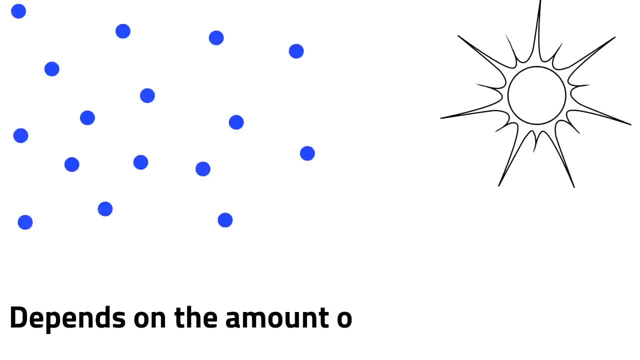 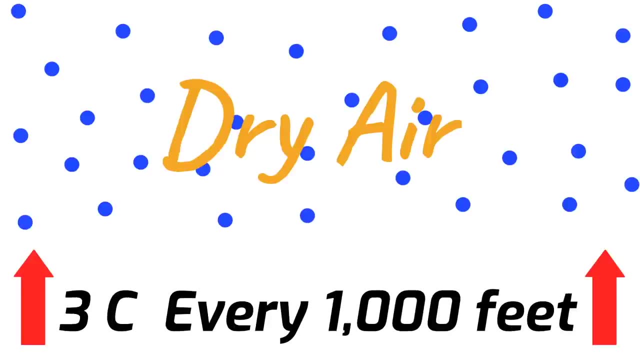 quickly the temperature drops depends mainly on how much moisture is in the air As it rises. if the air is completely dry, it'll cool off about 3 degrees Celsius every 1,000 feet of altitude that it goes up, And if there's any moisture in the air it cools off even slower. 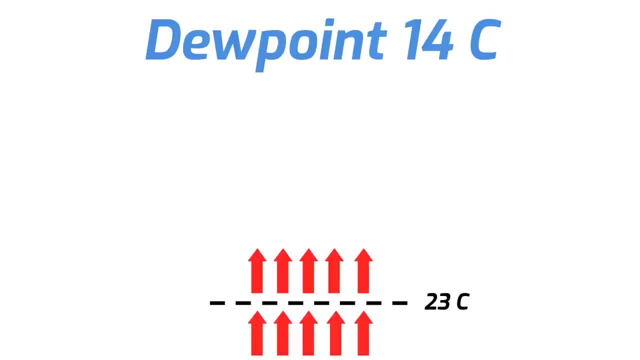 than that. That means that as that warm air rises, it cools and gets closer to its dew point. That's why clouds typically form high in the sky. With that in mind, we can actually estimate the height of the clouds if we know our temperature and dew point. 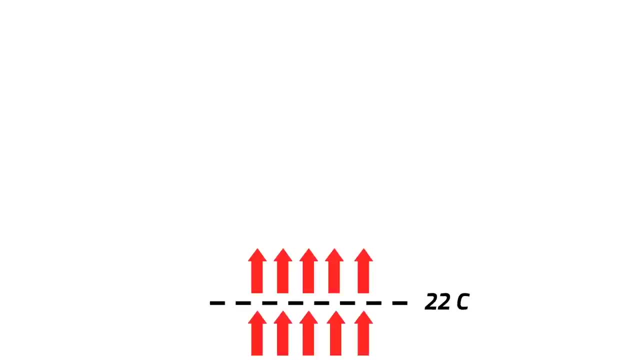 So now we know that as that warm air is lifted, it cools at a certain rate, depending on how much moisture is in the air. In addition to that, as that warm air is cooled, it can't hold as much water vapor either, so the dew point decreases as well. But it doesn't decrease quite as quickly as the temperature does. So as altitude increases, temperature and dew point get closer together or converge, And the rate at which it does this is 2.5 degrees Celsius. And remember, any time you see the temperature equal the dew point. 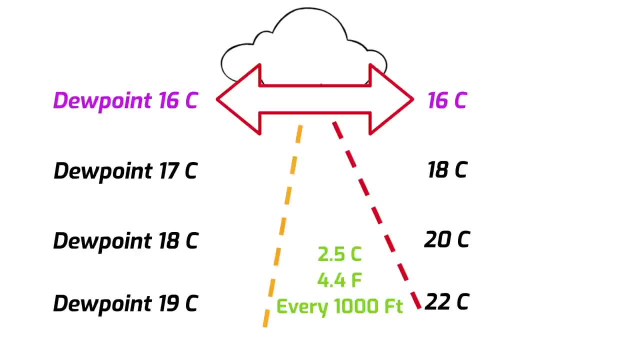 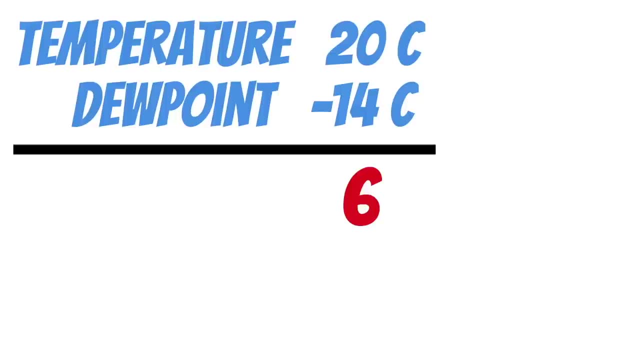 that's where you're going to see the clouds, rain, fog and all kinds of other moisture. So now that we know that we can take the temperature and subtract the dew point, and then you can actually divide that by the convergence rate of 2.5 degrees Celsius, 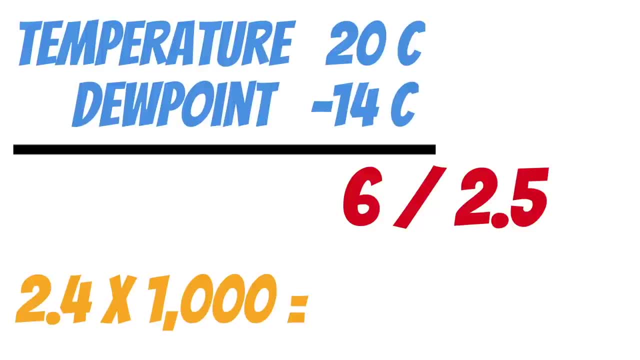 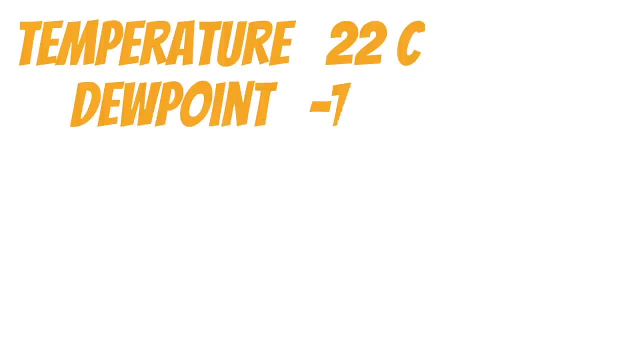 Then all we have to do is multiply that times 1,000 feet, and that's where the base of our clouds should be. Here's another example: Let's say our temperature is 2.5 degrees Celsius, The temperature is 22 degrees Celsius and our dew point is 18.. 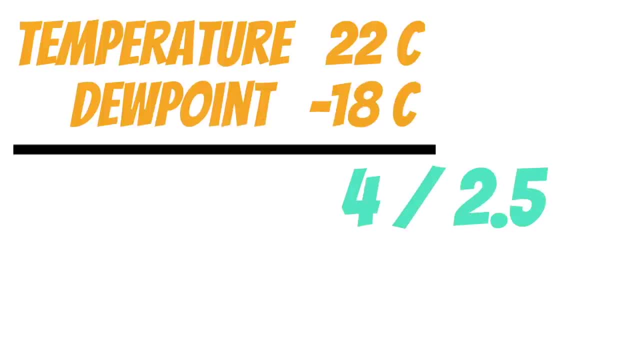 22 minus 18 is 4.. And 4 divided by our convergence rate of 2.5 is 1.6. And 1.6 times 1,000 is 1,600.. So in this example, the base of our clouds start at 1,600 AGL. 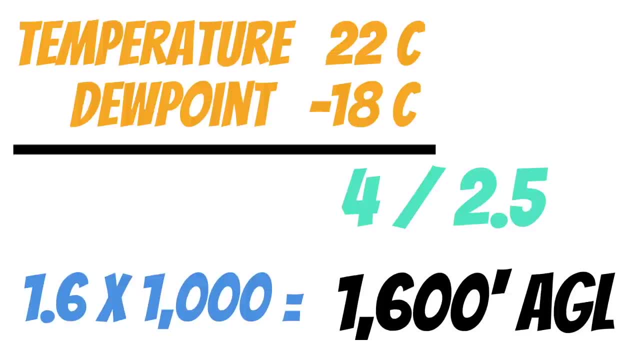 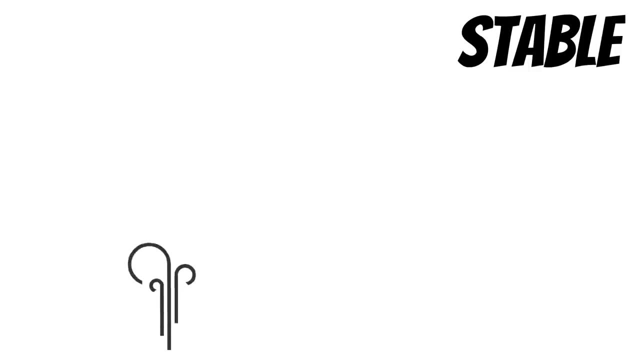 And this can change slightly depending on how stable the air is in that area. Stability is the atmosphere's ability to resist vertical motion. When the air is stable, if there's a minor disturbance in temperature and pressure, these small disturbances will get smaller and smaller. 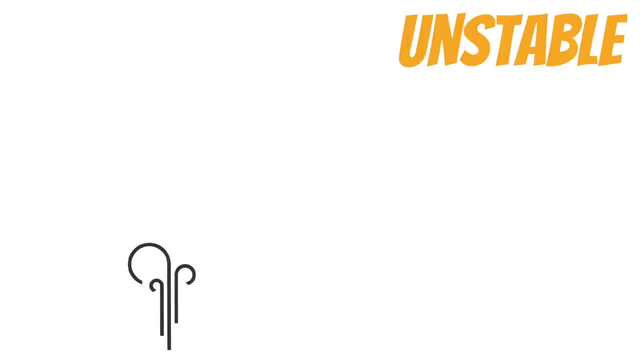 until they completely disappear. When the atmosphere is not stable, these small disturbances will get bigger and bigger, and that warm air will rise faster and faster. Temperature and moisture are the biggest contributors to atmosphere stability. The hotter the air is close to the ground, the faster it'll rise. 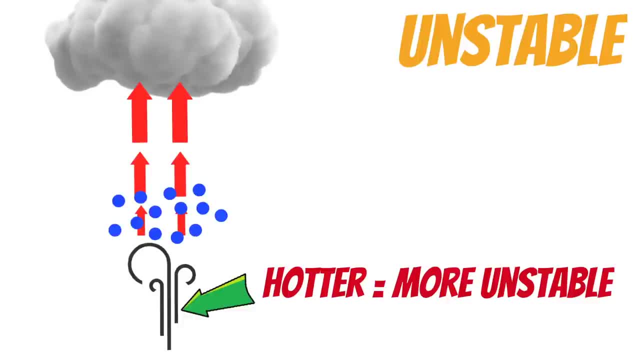 And the hotter the air, the more water vapor it can hold, And because water vapor is actually lighter than air, this can cause warm air to rise up even faster if it's got a lot of air in it, And that's why we're going to talk about. 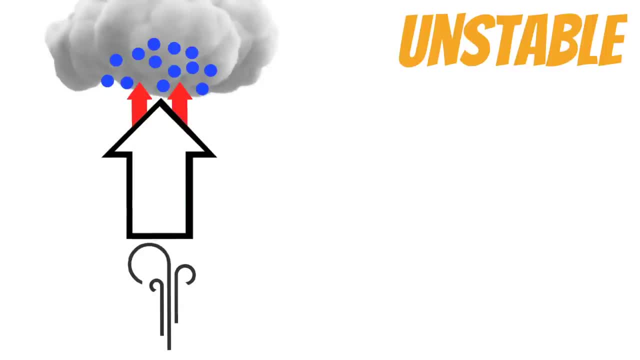 thunderstorms and other convective weather, And the faster that air moves upward, the more violent the weather can get. This is why thunderstorms and other convective weather is so common in hot, moist areas, And the more moisture that is added to the air, the more unstable this air gets. 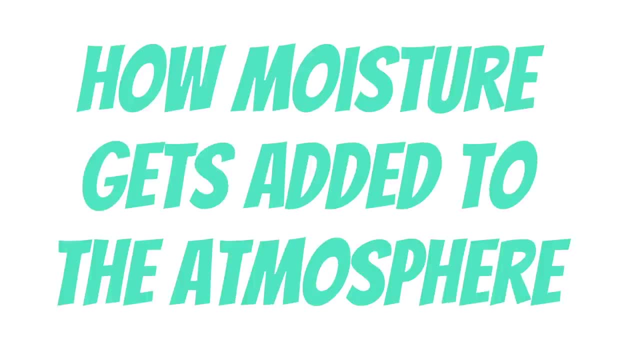 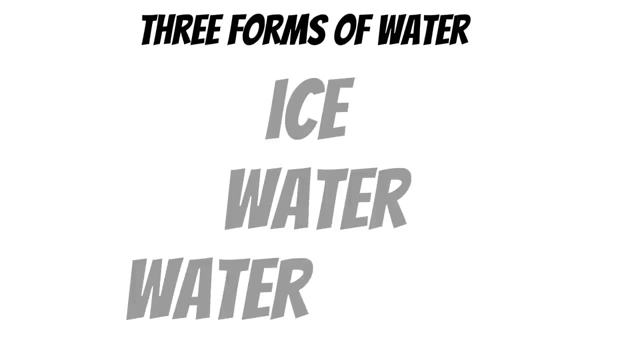 And, with that in mind, moisture can be added to the air in a few different ways. Now, as you probably already know, there are three forms of water in our atmosphere- solid, liquid and gas- And they can easily change forms to either. 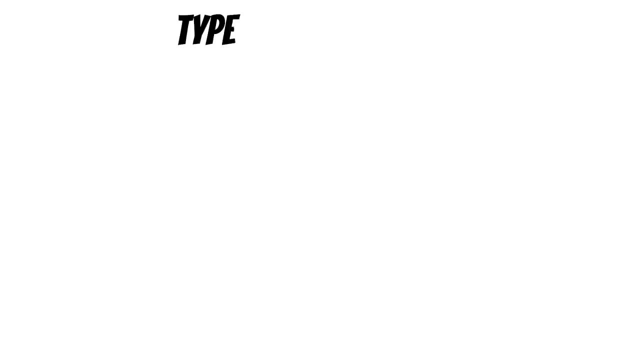 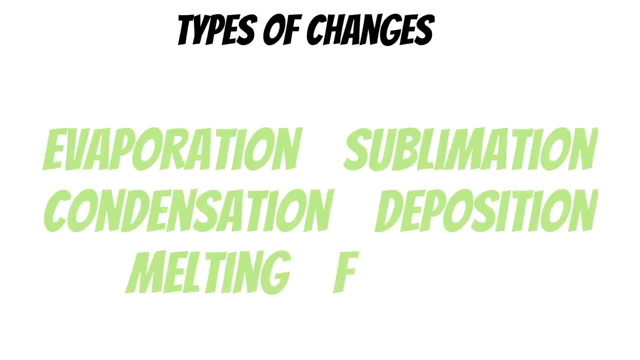 any other form when a heat exchange takes place. These are the different types of changes that can take place: Evaporation, sublimation, condensation, deposition, melting or freezing. But to understand today's concept, the only two you need to be familiar with is evaporation and sublimation. 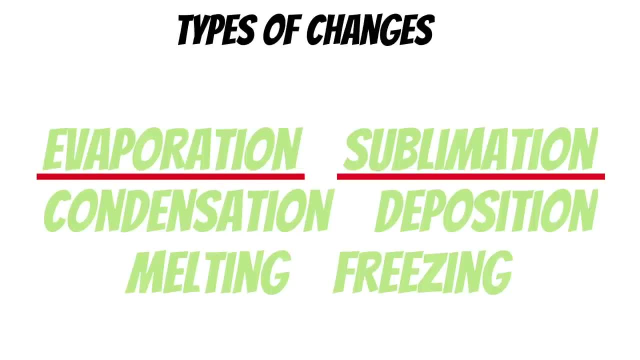 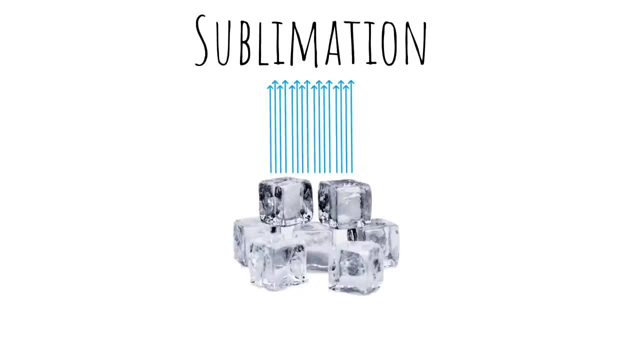 These are the only two ways that water vapor can be added to the atmosphere. Sublimation is when the solid form of water changes directly into a vapor. This process is a little less common than evaporation, because it requires a drop in air pressure as well as an increase in temperature. 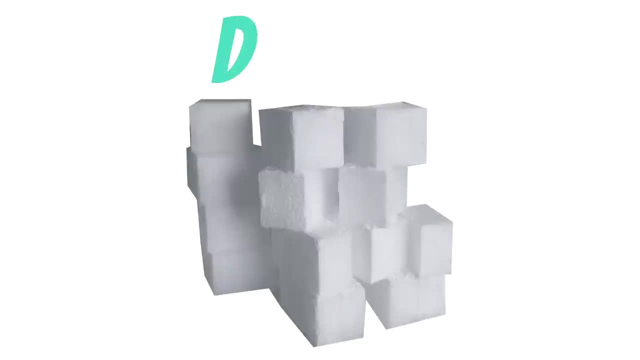 When I think of sublimation, I think of dry ice. Now, dry ice isn't really the solid form of water, but the process that happens when you heat it up is really similar. Evaporation, on the other hand, is the primary process that water vapor is added to the air. 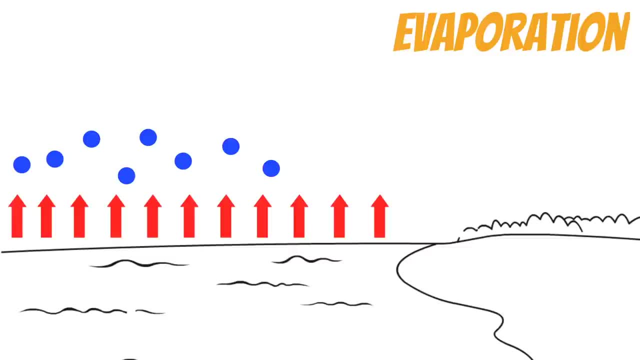 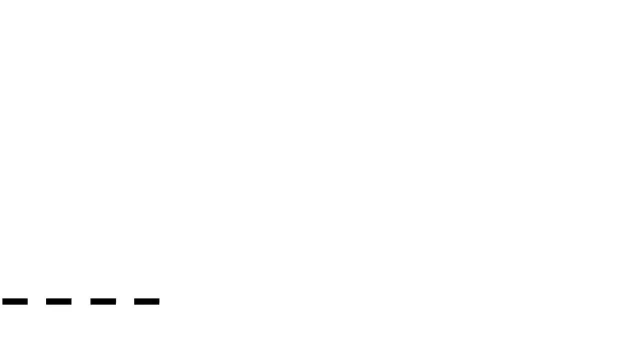 And the hotter it is, the more quickly water evaporates, And the more quickly it evaporates, the more moisture is in the air, And that makes the air even less stable. In addition to all that, sometimes the temperature doesn't always drop. 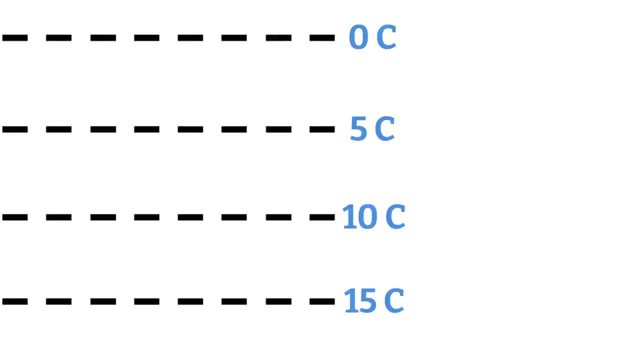 exactly 2 degrees Celsius every thousand feet. If the temperature drops faster than that, the warm air can rise even more quickly, And once again, this would mean that air is even less stable in these areas If the air temperature changes more slowly than 2 degrees for every thousand feet. this would make the atmosphere more resistant to upward or downward movement. In fact, it's also possible for the air to get warmer with altitude, and this is called a temperature inversion. When this happens, any moisture in the air can get trapped close to the surface. 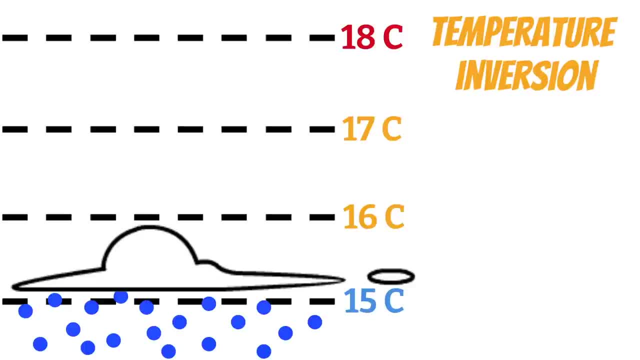 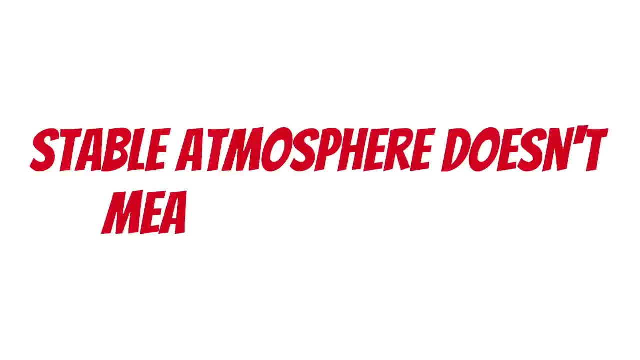 This can mean low clouds, fog, haze, smoke and other types of poor visibility situations, And this is where a lot of students get confused. A stable atmosphere does not necessarily mean good weather. It means that you don't have a lot of upward and downward movement of air in these areas. 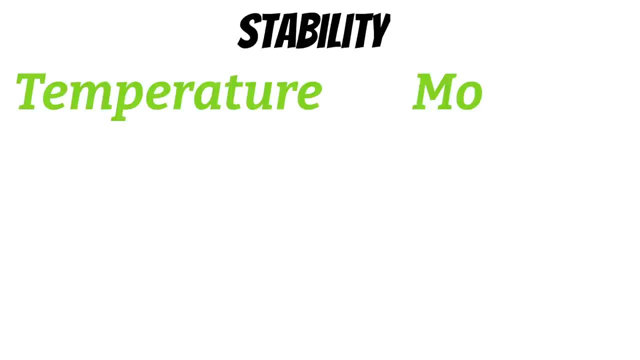 And the stability of the air, in conjunction with the temperature and moisture, are what determines what types of clouds, wind or atmosphere to appear and move through clouds. you see Now, clouds are primarily broken up into four categories: Low clouds, middle clouds. 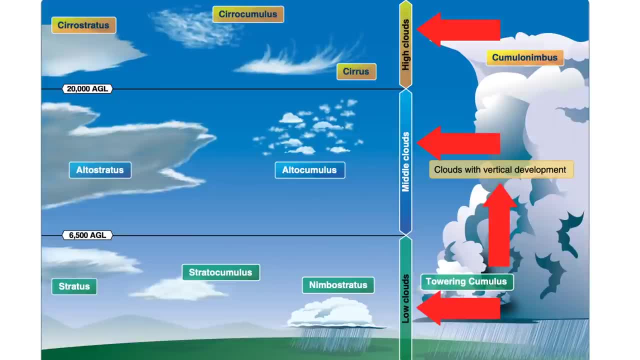 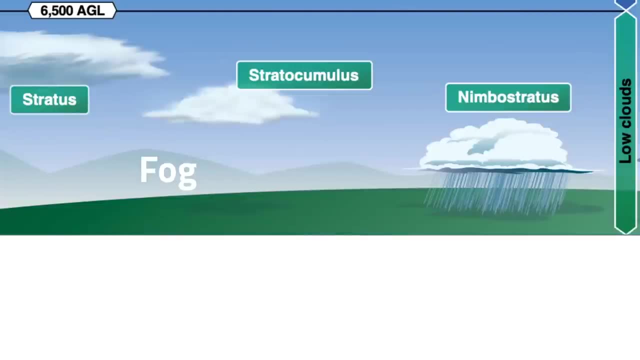 high clouds and clouds that span all of these. because of vertical development. Low clouds can be anything from fog, stratus, stratocumulus and nimbostratus. These form near the surface and extend to about 6,500 feet AGL. And these are of particular importance to you because these are 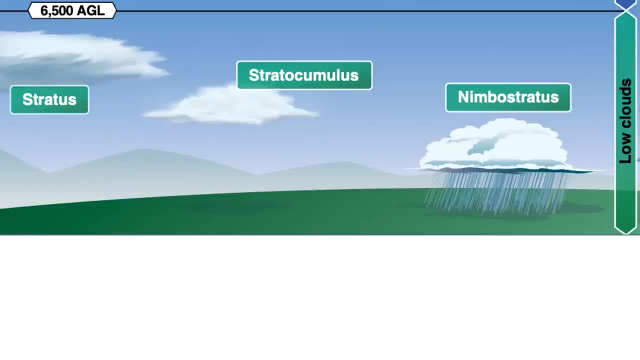 going to affect your ability to fly under visual flight rules. Here's some examples of some low clouds: Stratus clouds are typically flat sheet-like clouds. Cumulus clouds are the puffy, friendly looking clouds. So these stratocumulus are just a mix of the two, And anytime you see nimbo or nimbus. 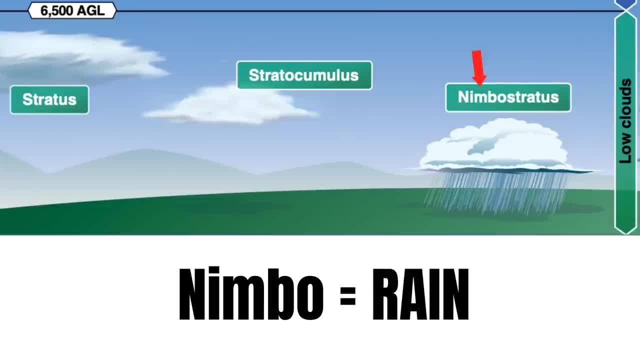 that just means it's a rain cloud or it has rain in it, And, once again, it's not uncommon to see any of these low type clouds when the air is stable, And that includes those nimbostratus clouds that have light, steady rain. 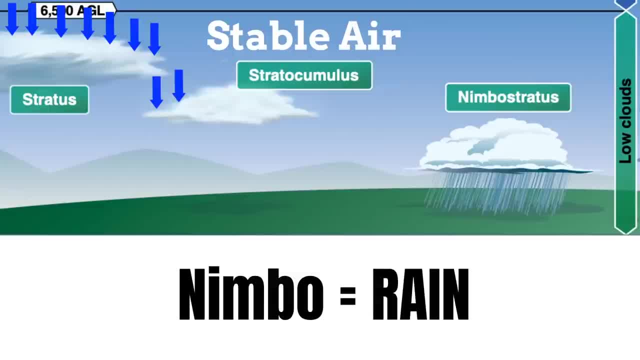 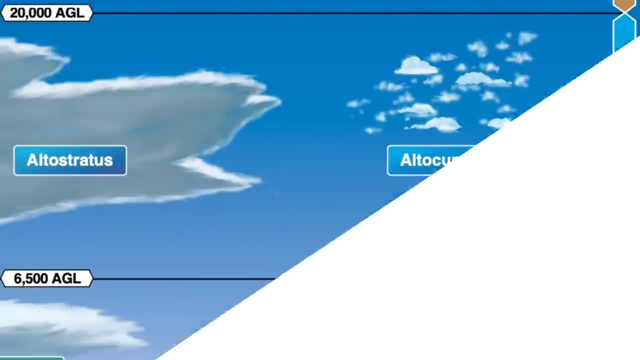 And that's because that stable air resists vertical motion, which keeps those clouds close to the ground. They're probably going to try to trip you up on the test with that question. Next, we have middle clouds. These typically form between 6,500 and 20,000 feet AGL. Typically, these come in two. 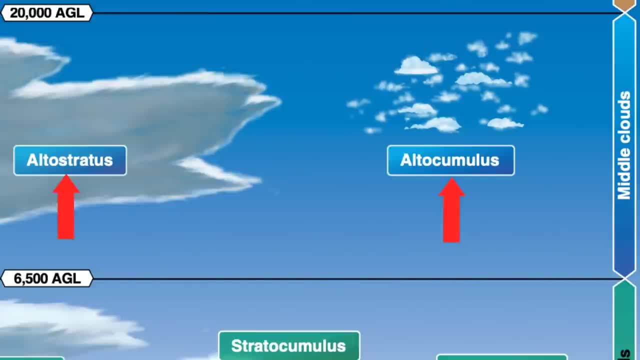 types: Altostratus and altocumulus. In altostratus clouds, you'll often find areas of turbulence and even areas of moderate icing. Altocumulus clouds may also contain a lot of air. So if you're looking to maintain areas of light turbulence and light icing- And these things are important to remember when you start working on your instrument rating and you start flying through clouds- 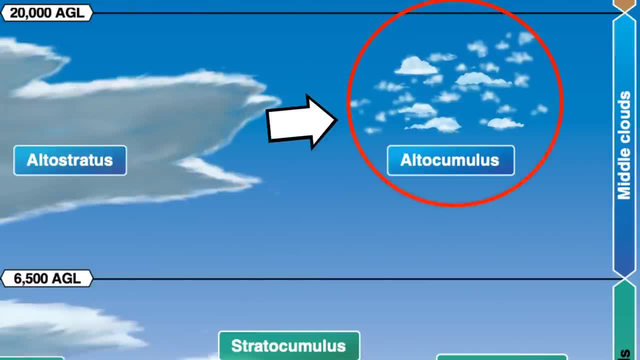 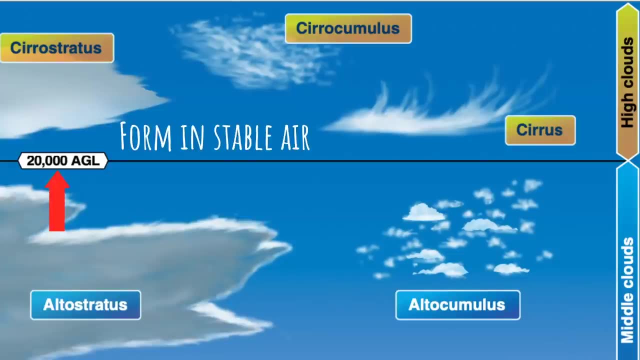 Altocumulus clouds are usually formed. when altostratus clouds break up, High clouds usually only form in stable air. These form above 20,000 feet AGL. Up here you'll find cirrostratus, cirrocumulus and plain old cirrus. These are these wispy ones. Then, last but not least, we have clouds with extensive vertical development. 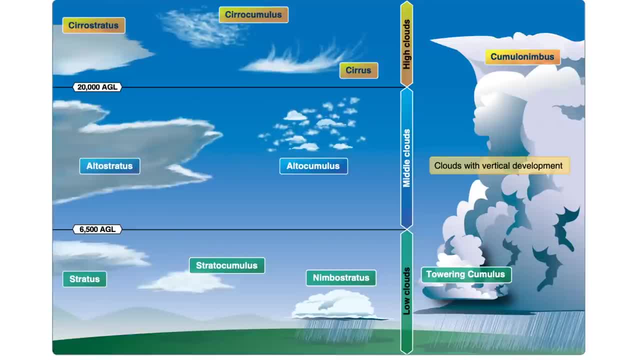 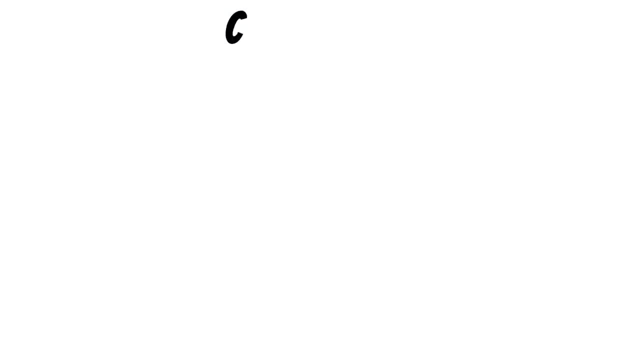 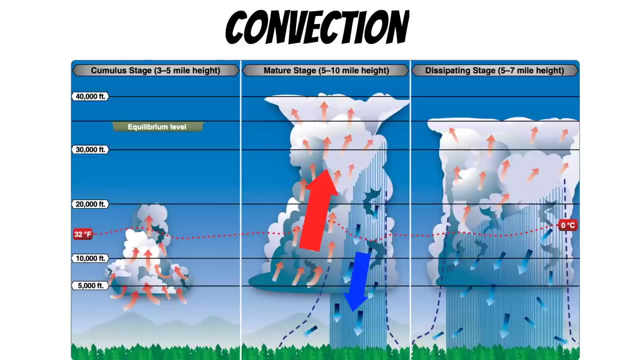 The bases of these typically form in the low to middle range, And these contain lots of warm, moist, unstable air, which rises very quickly. as we said before, This is what we call convection. In addition to these updrafts, air that cools is brought back down, along with air that's cooled by precipitation. 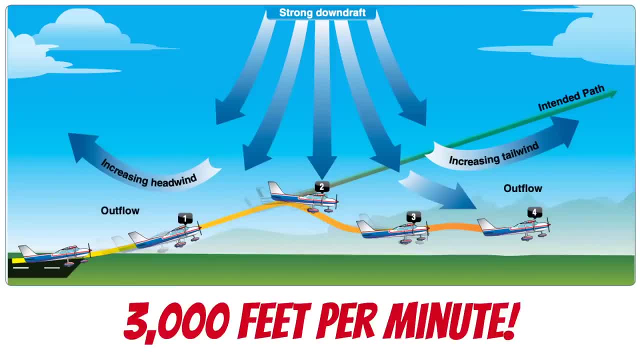 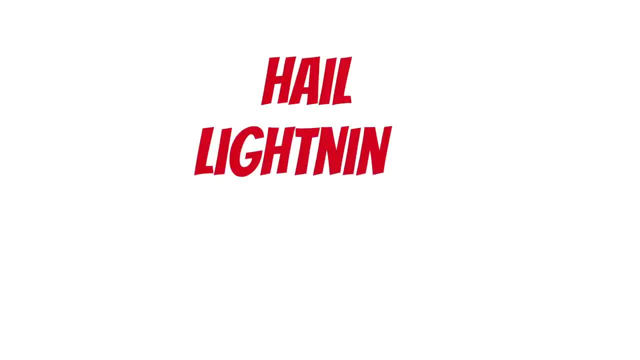 This can cause downdrafts in excess of 3,000 feet per minute, And this is one of the most dangerous parts of a thunderstorm. But in addition to that, thunderstorms can produce hail, lightning, tornadoes, heavy rain and all kinds of scary stuff that I don't want to fly in. 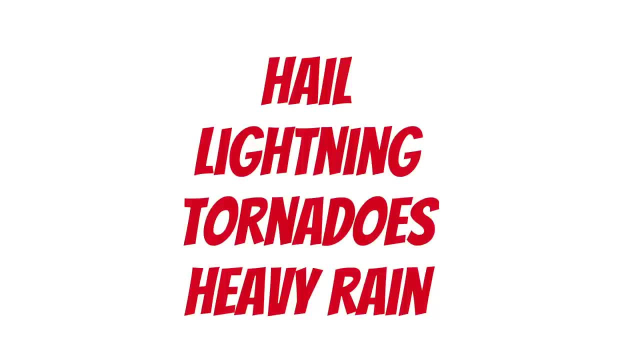 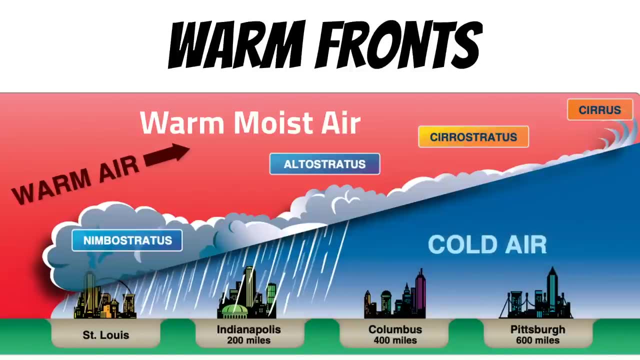 So now that you have a good understanding of that, let's go back to talking about fronts, And we left off talking about warm fronts and how they bring a lot of warm, moist air into the area, And when any front moves into an area, the weather you get depends on how stable the air in that area was before that front moved in. 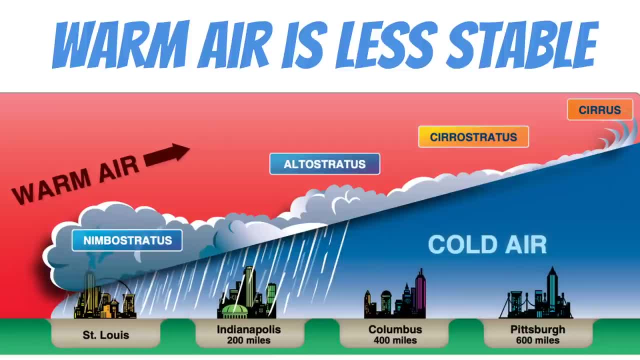 Remember, warm air is less stable because warm air rises And it holds more moisture, which makes it even less stable. Now, in almost all atmospheric conditions, this is typically the type of cloud conditions that you'll see with an approaching warm front. 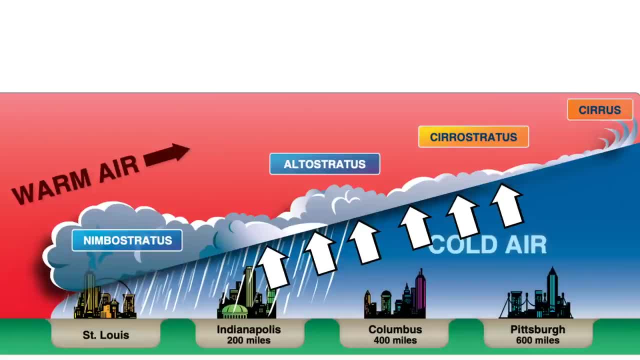 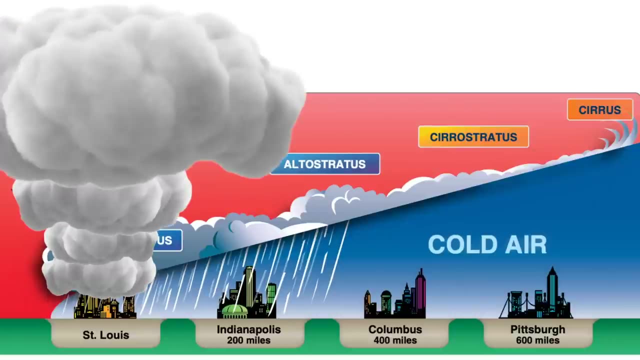 Before it hits, you'll usually see these flat stratus-type clouds which roughly follow the bottom edge of that warm air. And the weather you get right here at the base of the warm front depends on the stability of the air, And if the air is unstable, which is typical of the summer months, you could see thunderstorms develop in these areas. 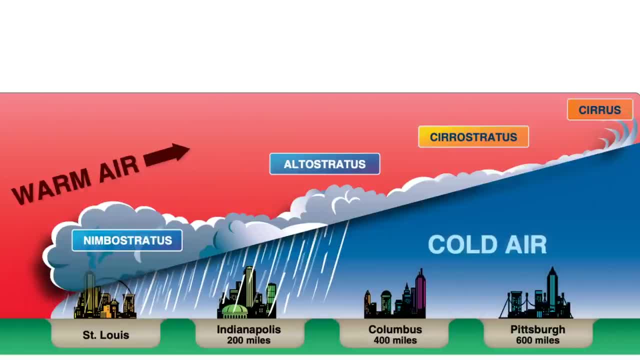 With that in mind, no matter how stable the air is, you can still expect to see drizzle or steady light rain in these areas. Visibility might be bad right before the front passes, but once it does, it can often get really clear outside, because that warm air can pick up a lot of contaminants and carry them away from the surface. 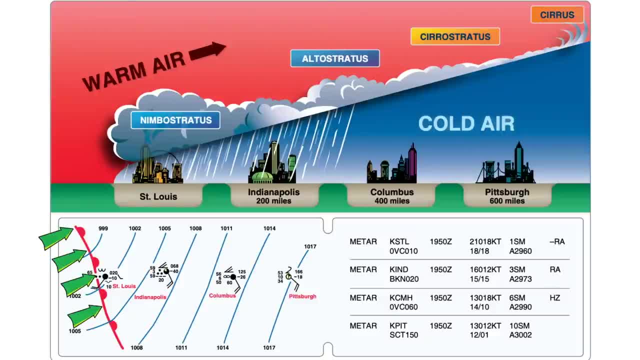 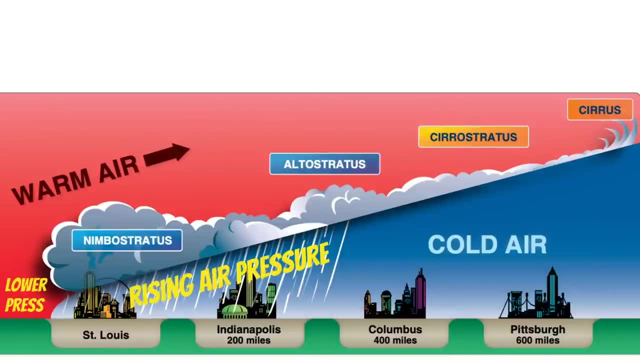 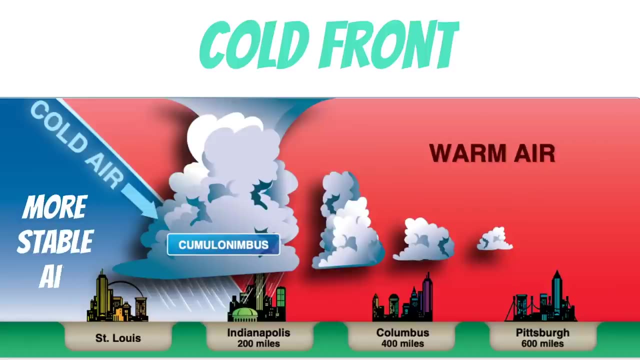 Also, as the front passes, expect the wind to change directions. And right before the front passes, the air pressure can rise slightly, And once it does, the pressure should go back down. Next we have the cold front. These are large air masses that are made of colder, denser and more stable air. 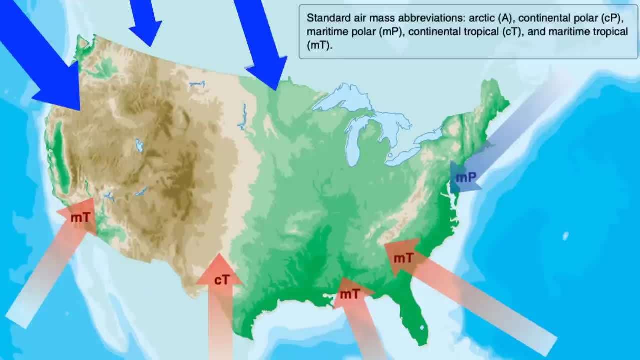 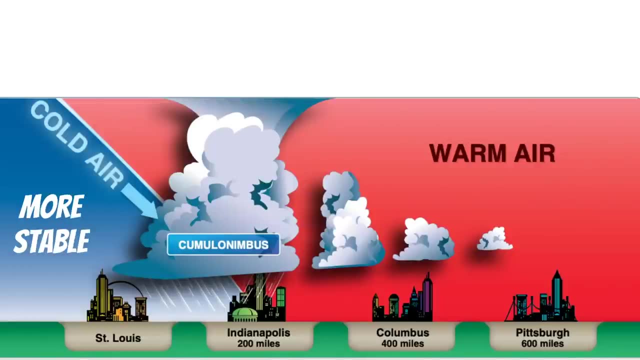 These commonly come from large areas of cold air in the Arctic and polar regions. Now, even though the colder air is more stable than the warm air, cold fronts move a lot faster than warm fronts, And they typically move about 25 to 30 miles an hour. 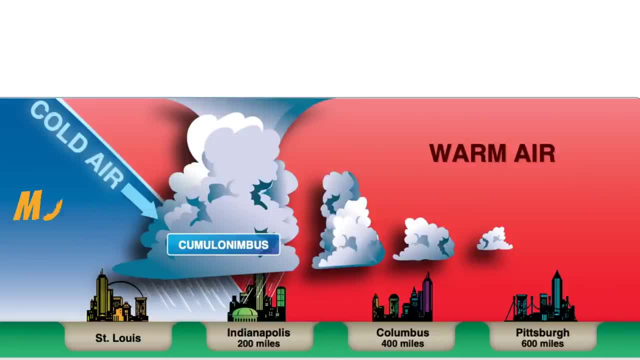 Okay, so we already know that the air inside of a cold front is more dense than the warm air in front of it, And this could be due to the fact that the air inside the cold front is more dense than the warm air in front of it. 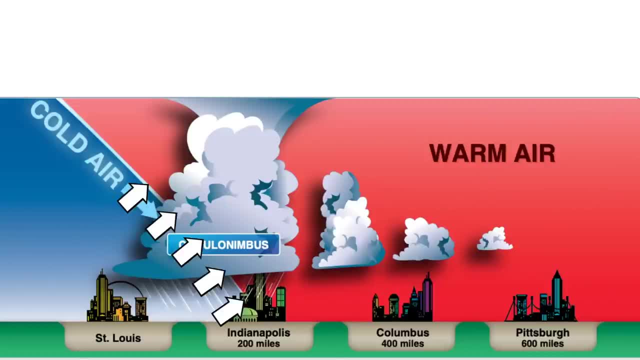 This causes the cold air to push that unstable warm air forward and up, which causes that lifting motion And that means that air right here is less stable And, once again, the type of weather that you get when a cold front passes depends on the stability of the air that was already there. 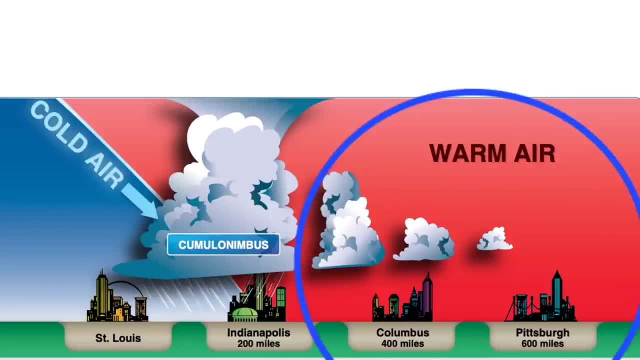 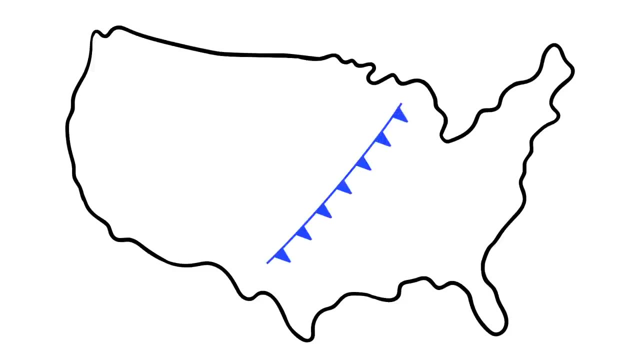 So during the summer, when the air is hotter and more moist, it's very common to see thunderstorms along the leading edge of a cold front, And cold fronts can be hundreds of miles long, And this can cause huge lines of thunderstorms at the beginning of the cold front. 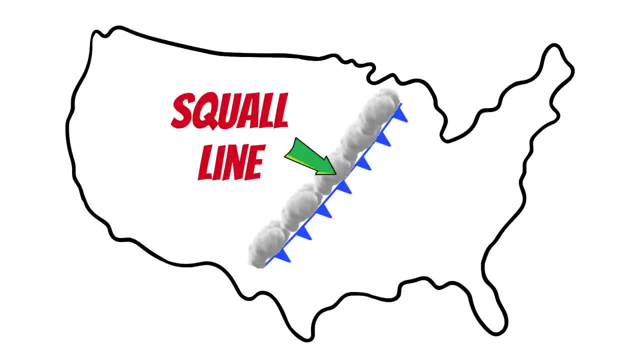 These are called squall lines. Right before the cold front passes, you'll usually notice a drop in air pressure because that warm air is being pushed up. You'll also find gusty winds coming from all different directions and poor visibility, And right before that cold front passes is when you can expect the worst kind of weather. 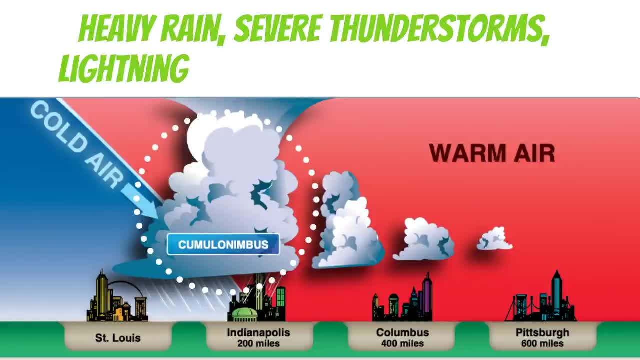 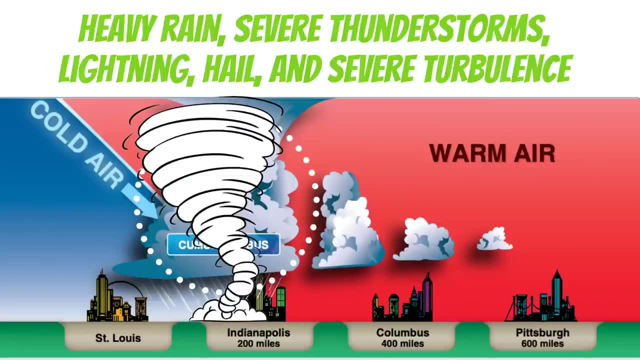 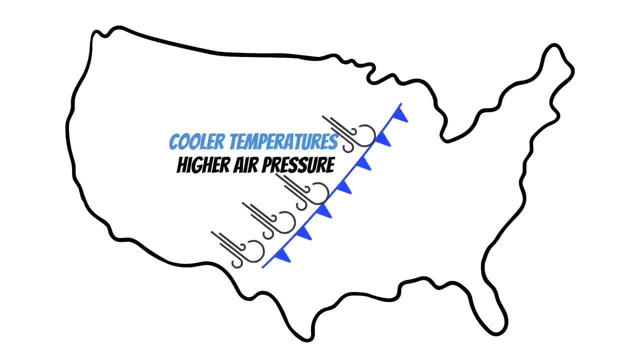 There can be anything from heavy rain showers to severe thunderstorms, with lightning, hail and severe turbulence. It's also not uncommon for cold fronts to produce tornadoes. Then, once the front passes, you'll usually see cooler temperatures, higher air pressure and winds typically flowing the same direction: the front is moving. 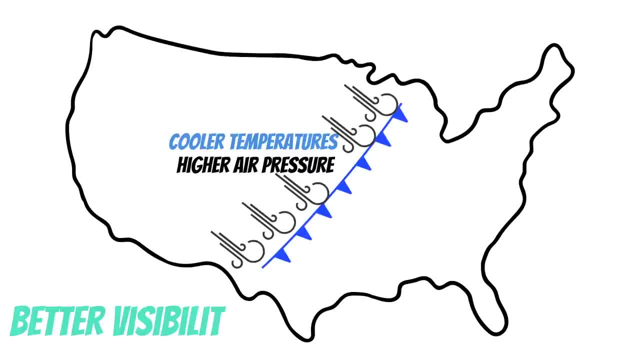 These winds usually help visibility improve as the front moves farther ahead. Now there is a possibility for a mixture of these two fronts to occur. If two opposing air masses meet each other and they're somewhat equal in strength, you'll get something called a stationary front. 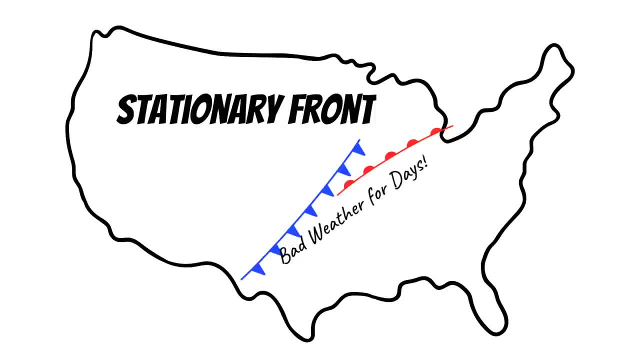 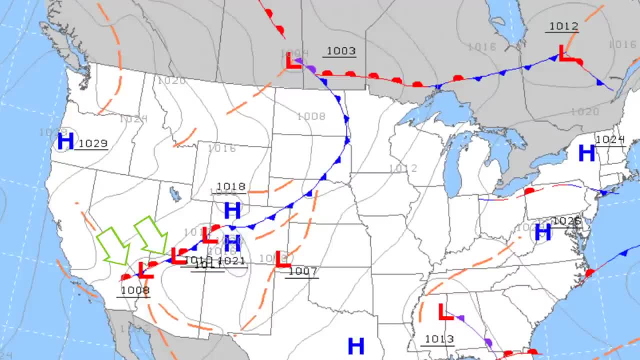 A stationary front can cause bad weather for days, and the weather you get is usually a mix between the weather you see in a cold front and a warm front. You can identify a stationary front on a weather chart by the opposing cold and warm front symbols. 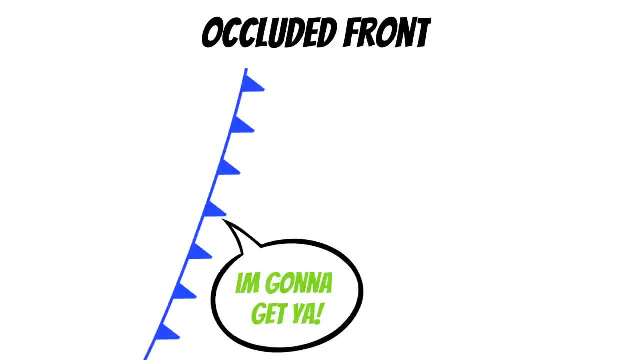 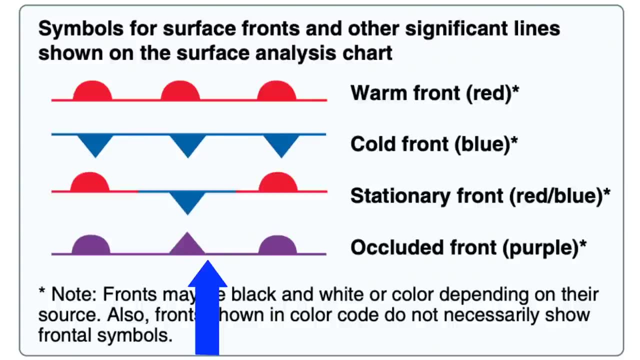 An occluded front, on the other hand, is what you get when a cold front catches up with a warm front. This is indicated on a weather chart by these purple lines with a mix of warm and cold front symbols. With an occluded front in the beginning, you can expect the same weather as a warm front. 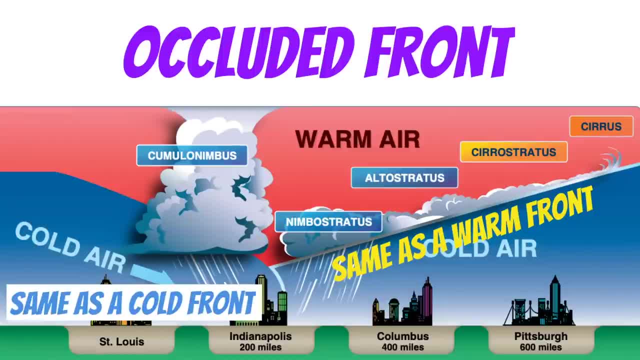 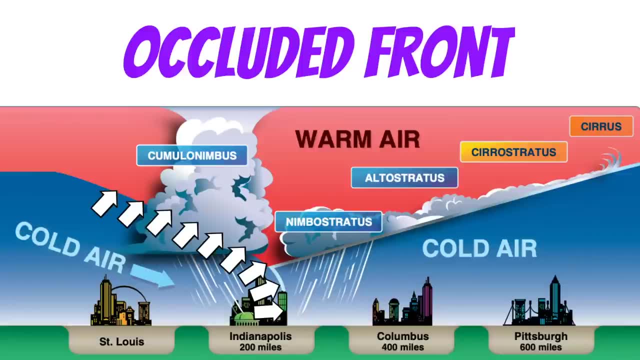 And this weather is immediately followed by the same weather that you would expect from a cold front. Typically, the cold front plows its way in and pushes that warm air from the warm front up and pushes the cool air that was there already straight ahead. 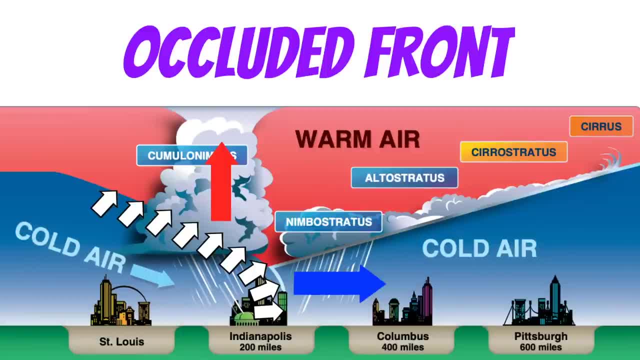 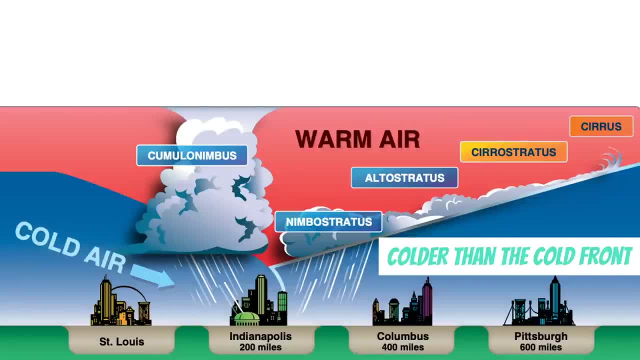 When it's able to push that cool air forward without any problems. this is called a cold front occlusion, But if, for some reason, that air that was already there is cooler than the air in the advancing cold front, this can cause some extremely violent weather. 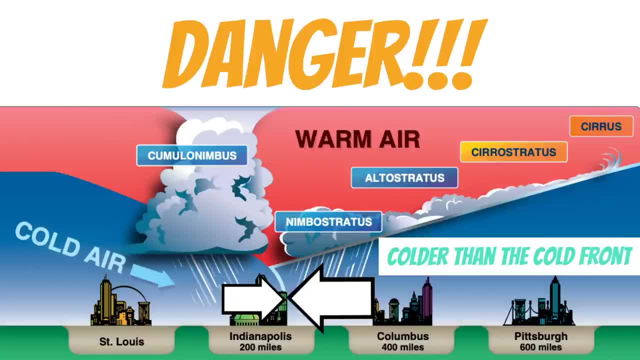 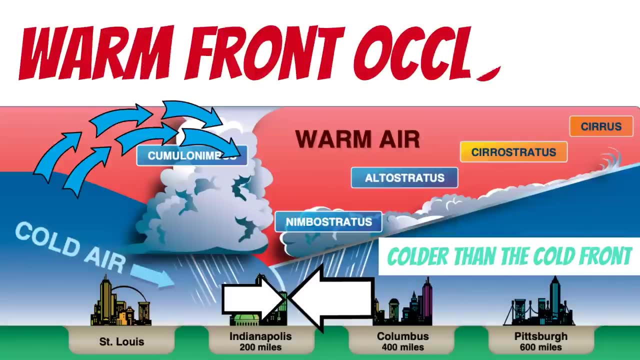 In this case, the cold front air can no longer push the cooler air forward, so instead it's pushed up over the warm front air. This is what we call a warm front occlusion, With this cooler air being pushed above the warm front air. this can cause extremely unstable lapse rates.